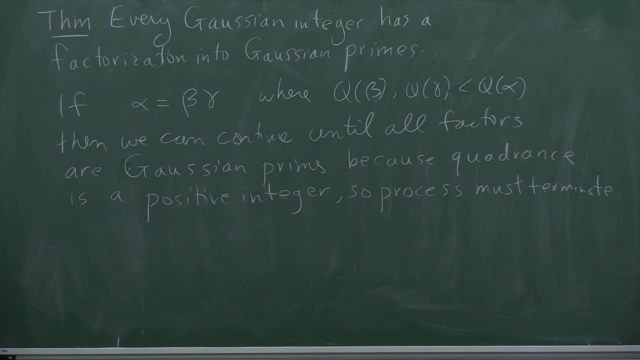 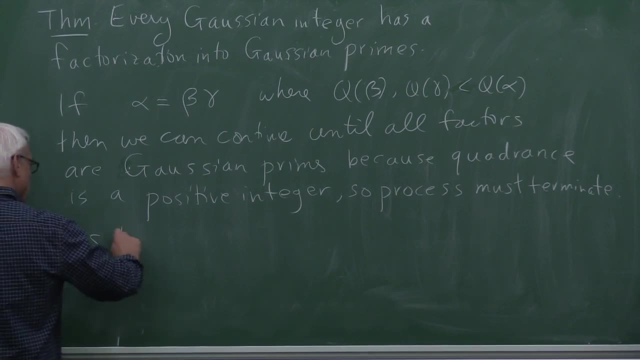 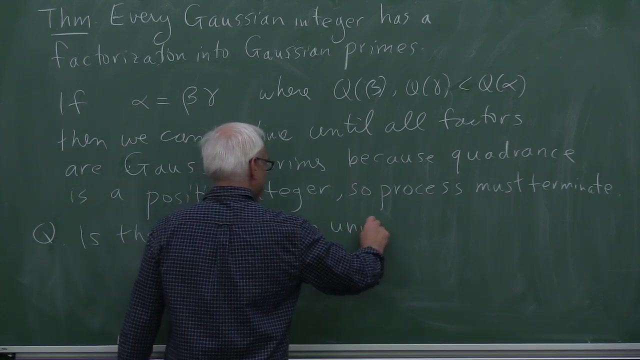 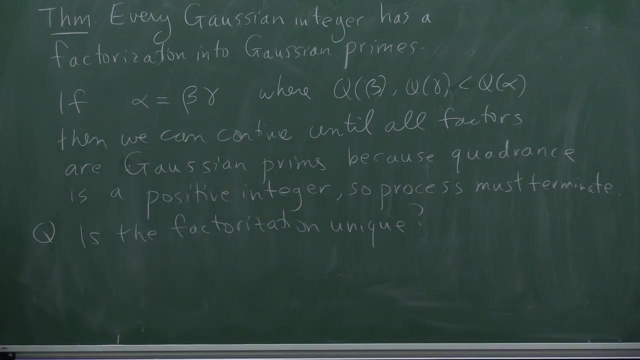 And we can continue until all factors are Gaussian primes. And we can continue until all factors are Gaussian primes. But is it unique? That turned out to be an important question. So the question is: is the factorization unique? Is it possible for a number to be a product of Gaussian primes in two quite different ways? 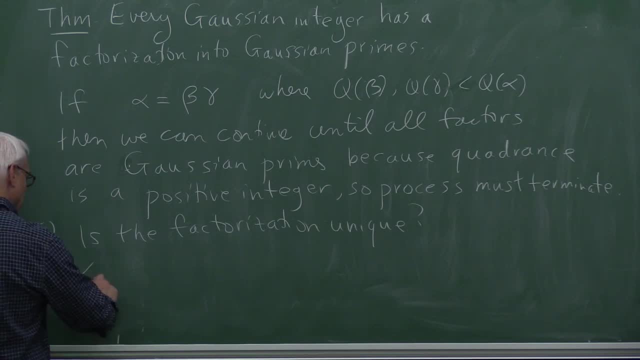 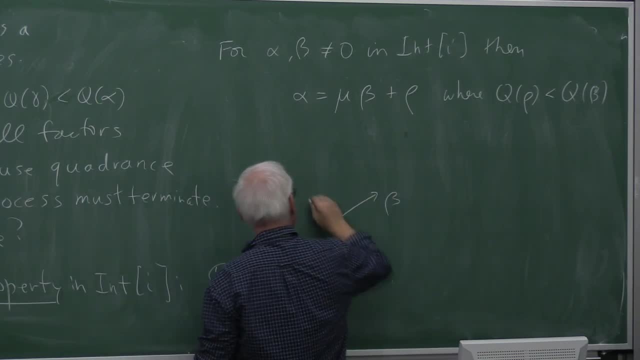 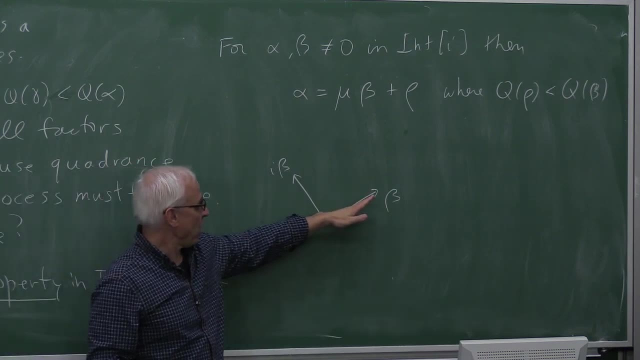 Well, it turns out that the number is a product of Gaussian primes in two quite different ways: complex plane here. Here is beta and here is i times beta. We have to know that when you multiply by i, the complex number rotates by a quarter turn and has the same size. So 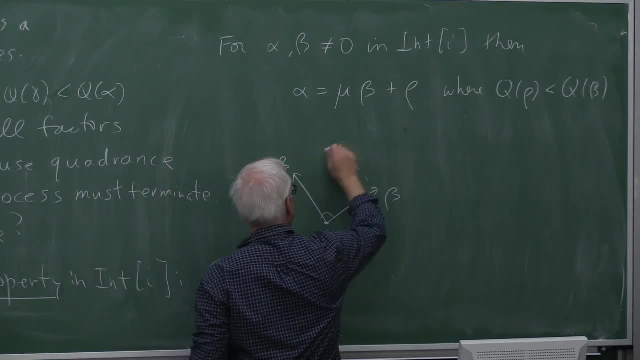 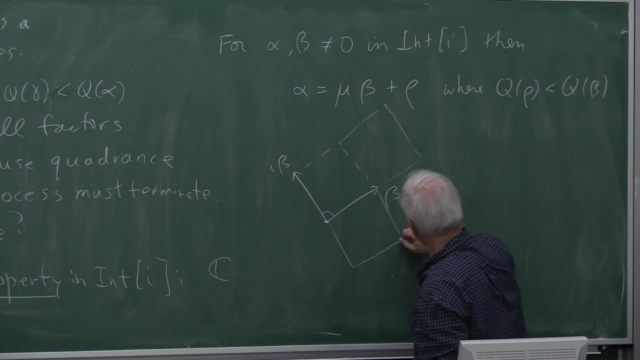 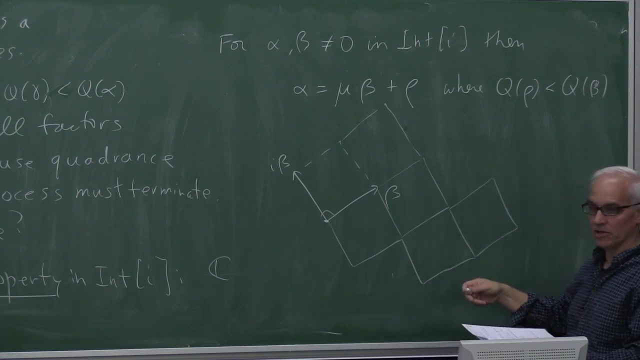 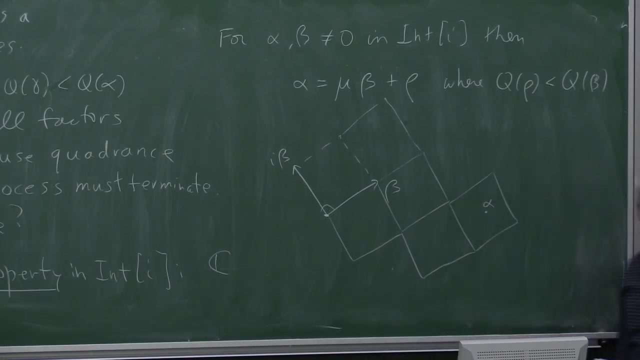 these will be perpendicular and they form a square. In fact, if we look at all multiples of beta, we get some square lattice in the plane. These are all integer multiples of beta and i beta. If we have some number alpha somewhere, then it's in one of these squares. 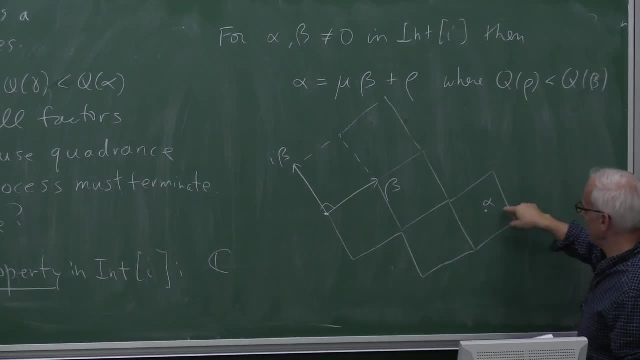 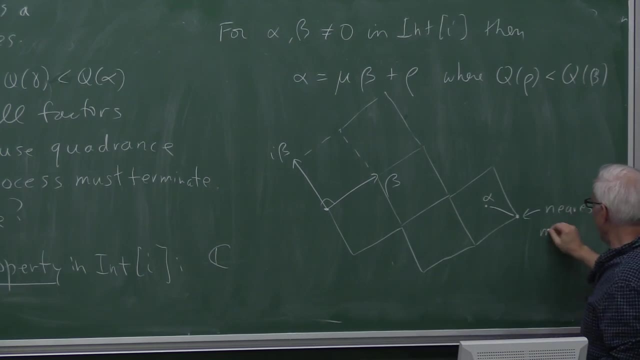 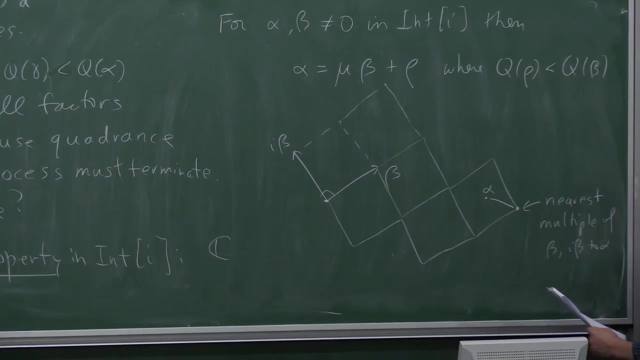 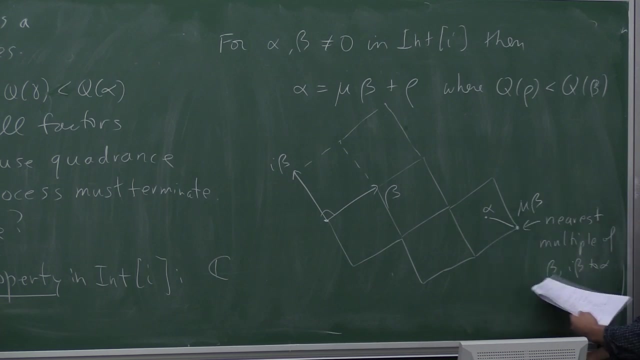 That means there's a nearest point in this lattice to alpha. Let's suppose that this is the nearest square, The nearest multiple of beta, and i beta to alpha. Let's call it mu beta. So if it's a multiple of beta, it's mu times beta for some Gaussian integer mu And this difference will. 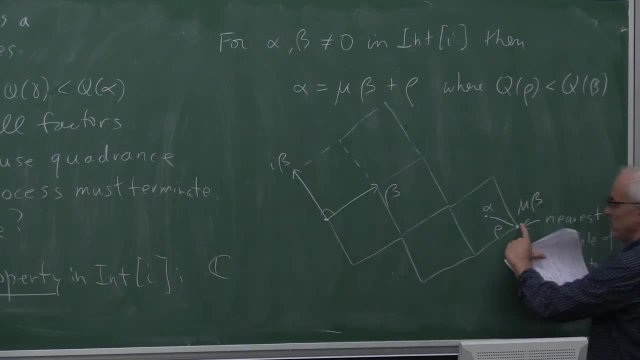 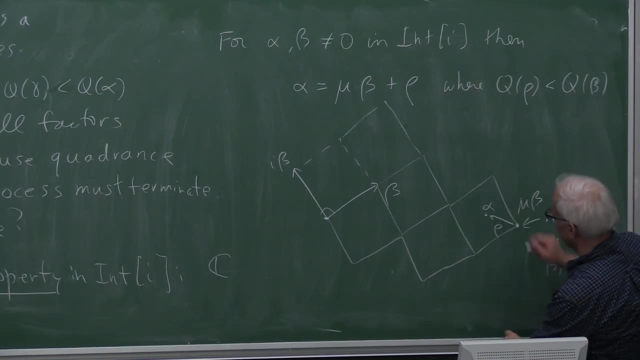 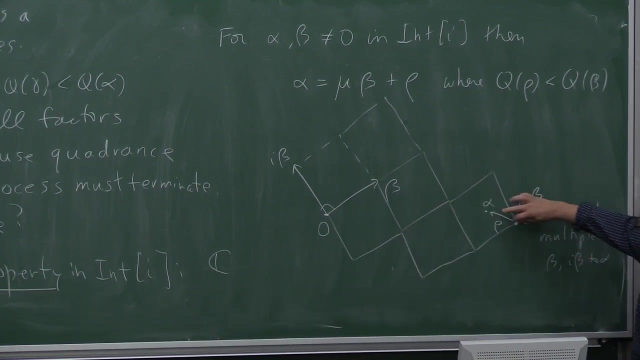 be rho. That's basically what we're saying: that alpha is equal to mu, beta plus some error. positive one minus beta, which is a pretty good thing, because it is not going to show up there, And what we have here now on the Y side is the traded product of this vector. We can. 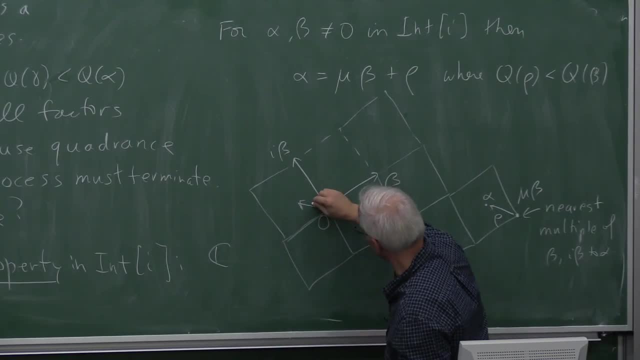 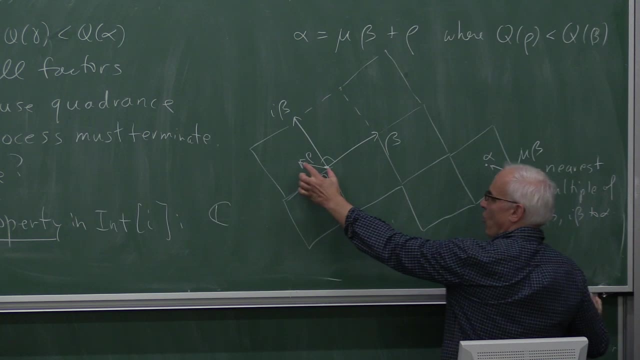 write this vector as 0 to the negative vai, And what this strangers me- is going to show up is a vector beta, which will beakh and beta, And this vector here is going to be comes from this Alam. that's just a littleл small vector from the zero, it's nothing. in the future. Let's come back to our 그림 and see what we can do to know if it is inflexible or not. Let's have an ordinary well to know, a logical example of that, and it is a really simple. 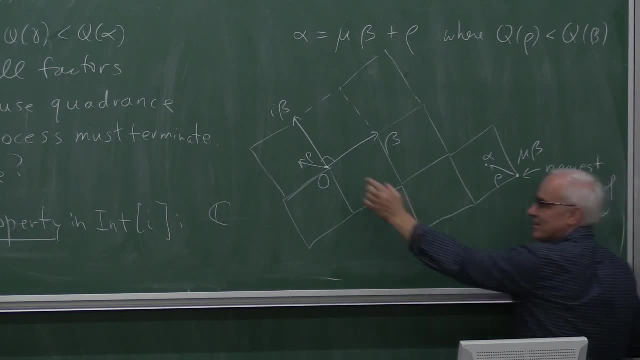 thing to use in this slide, This obrigittal equation. Therefore, we're going to be doing something like relating- So we're going to look at H- to a greater Hasselheim's equation, which, That's the statement that this difference is smaller in size than beta is. 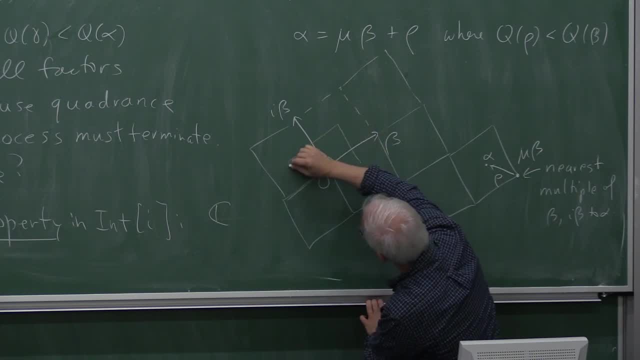 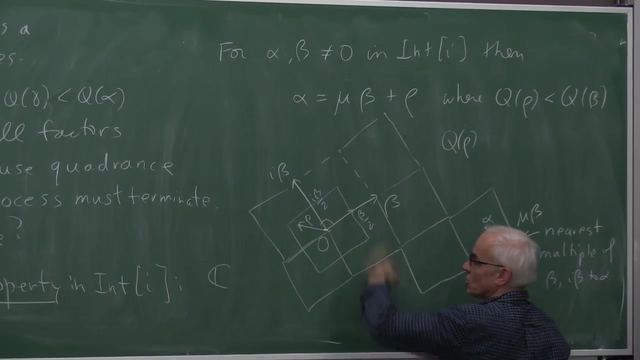 We can see that by observing that this rho has to be in the square here where this is beta over 2, and this is i beta over 2.. And so, the quadrants of rho being inside this square, it will be less than or equal. 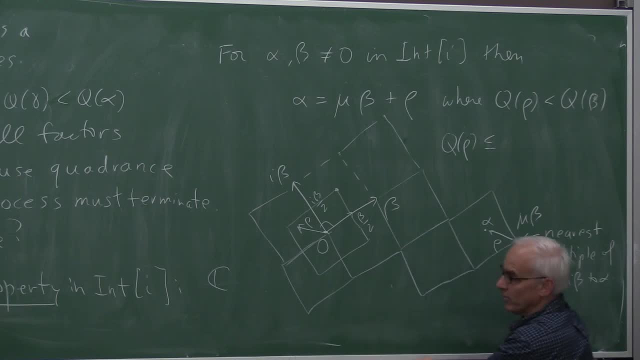 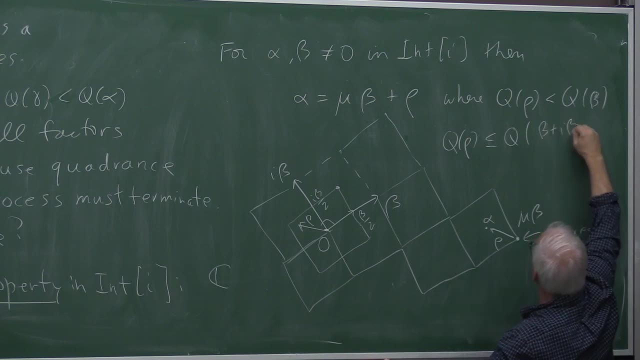 to the maximum possible value of the quadrants in that square, which will be this: quadrants of beta plus i beta over 2.. This is the point: beta plus i beta over 2.. And by the moment that we get to this point, we're going to be able to see that this is: 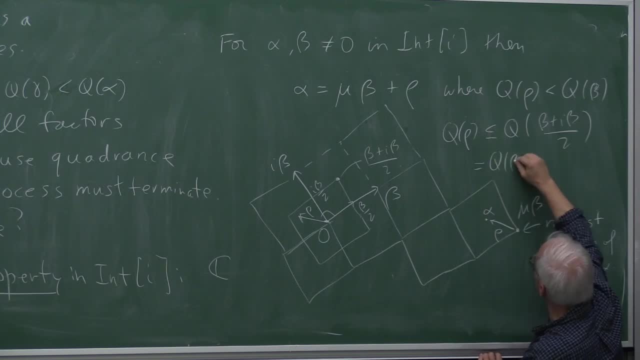 a multiplicative property of the quadrants. This is the quadrants of beta, times the quadrants of 1 plus i over 2.. And what is the quadrants of 1 plus i over 2?? Well, it's that times its complex conjugate. 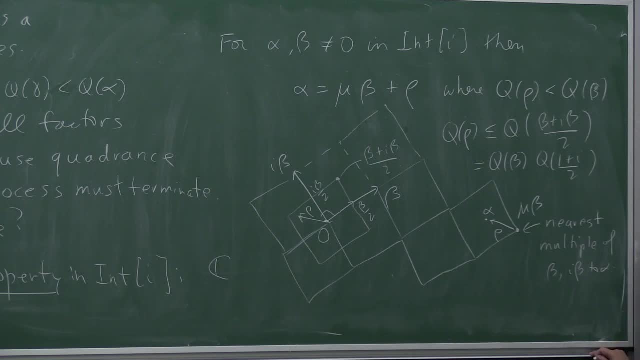 So it's 1 plus i times 1 minus i over 4.. That'll be 2 over 4, or 1 half, So this will be beta over 2.. Sorry, it'll be quadrants, Quadrants of beta over 2, sorry. 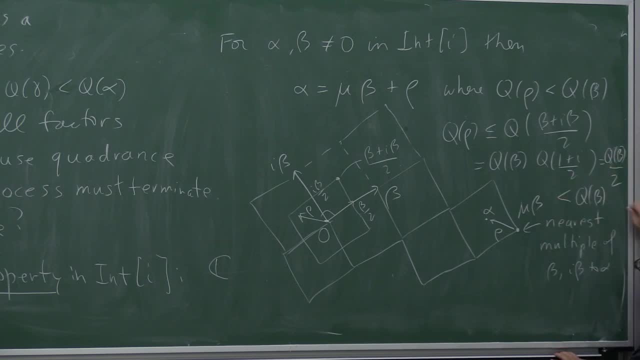 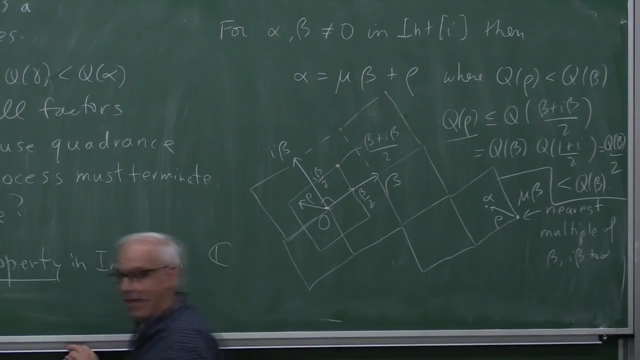 And that'll be less than the quadrants of beta. That's the crucial inequality: that the quadrants of rho is ultimately less than the quadrants of beta. Well, that makes the division algorithm work. And then, if you go back to the Euclidean proof of unique factorization, Euclid's proof of 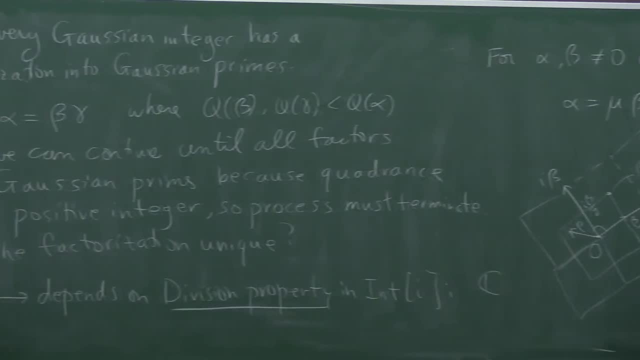 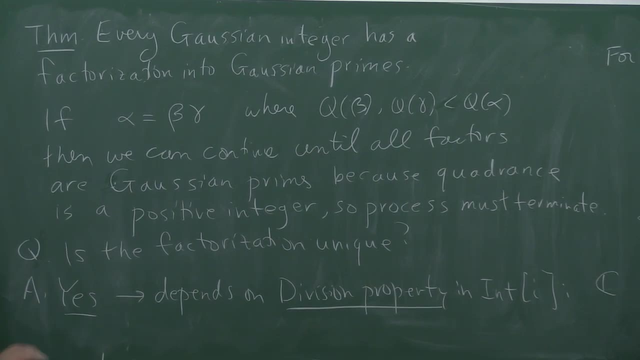 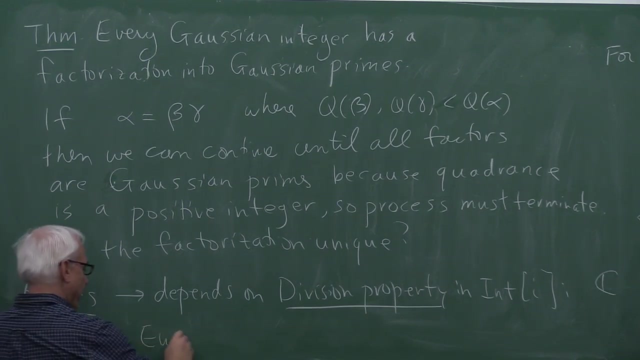 unique factorization. It basically employs this property crucially for the unique factorization. So then you can take that proof and just adapt it to this situation and it works. So the Euclidean proof essentially works here, Once we have this crucial division property. 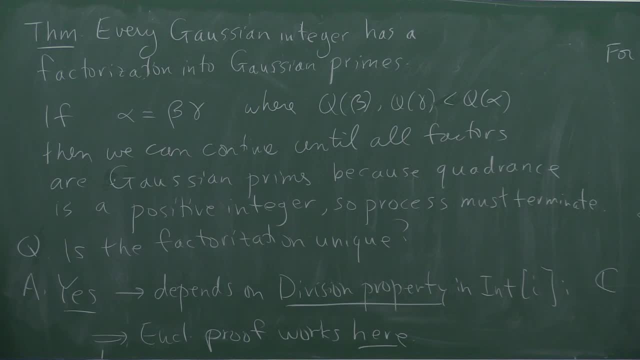 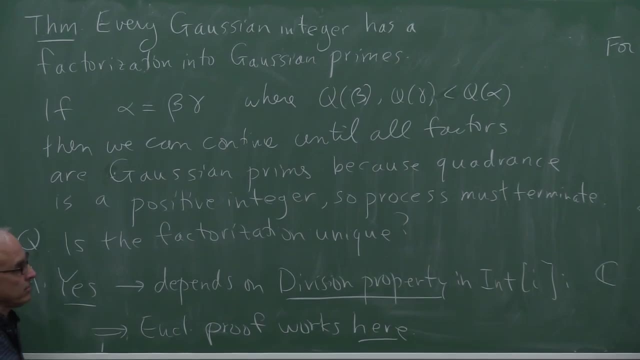 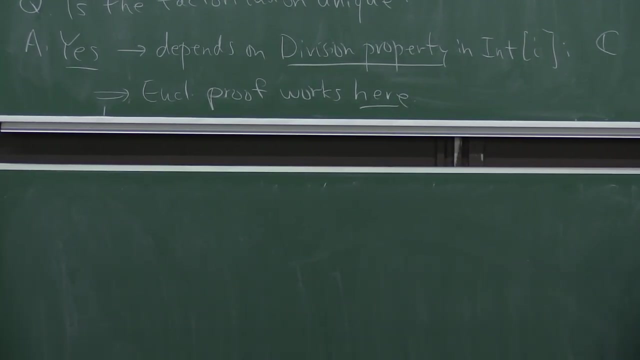 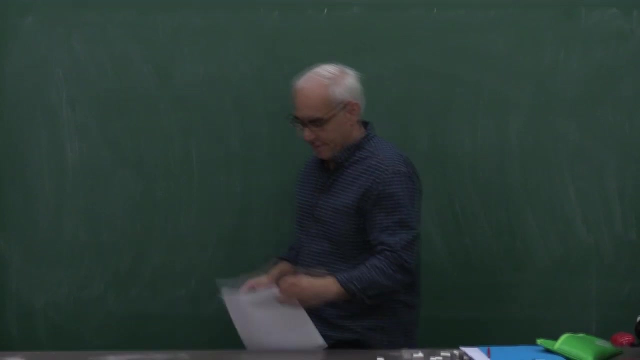 So, yes, it's true that in the Gaussian integers there is unique factorization into props. So people thought, well, that's great. This kind of arithmetic with these kinds of numbers is much like what we're used to. But, however, there was a shock in store. 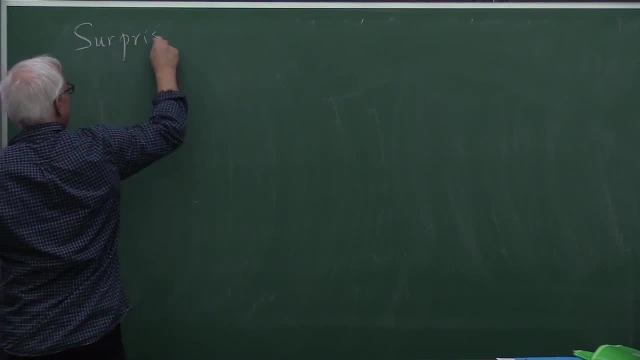 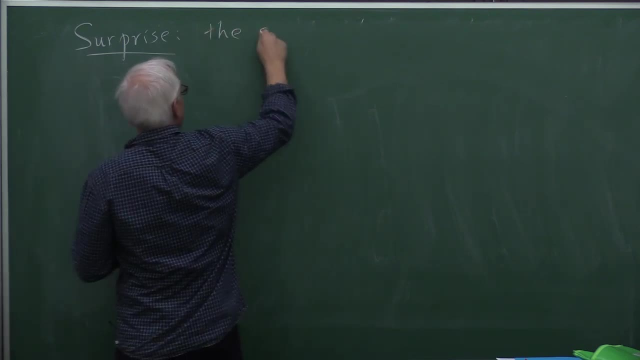 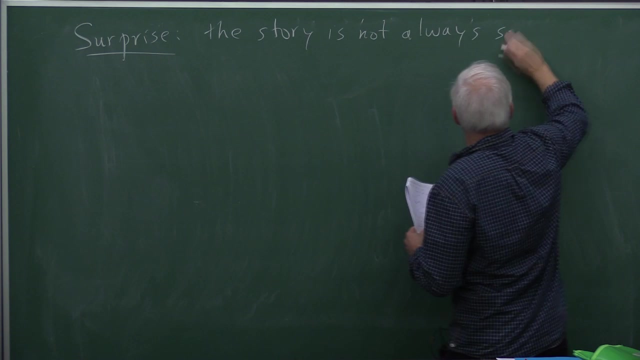 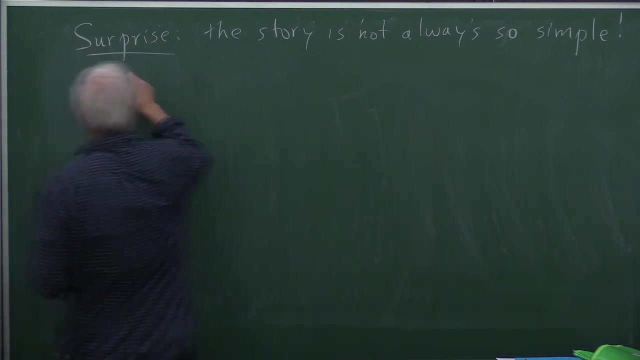 Okay, So there was a surprise. The surprise is that it's not always so simple. The story is not always so simple. So, in particular, if we look at The integer, The integer's adjoined square root of minus 5.. 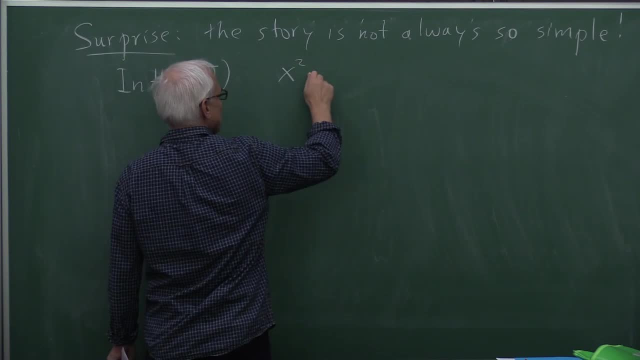 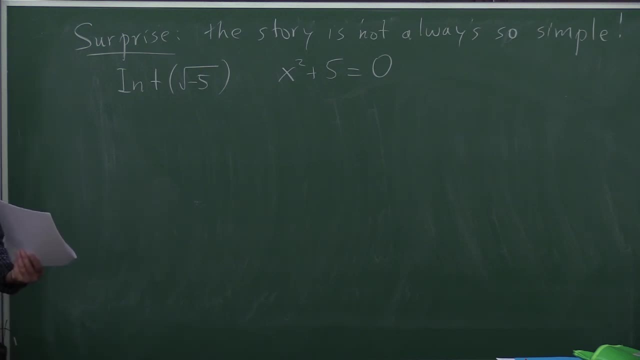 So here what we're doing is we're taking the equation x squared plus 5 equals 0. We're looking for solutions to that equation. If you're happy with complex numbers, you would say: well, that's the square root of minus 5.. 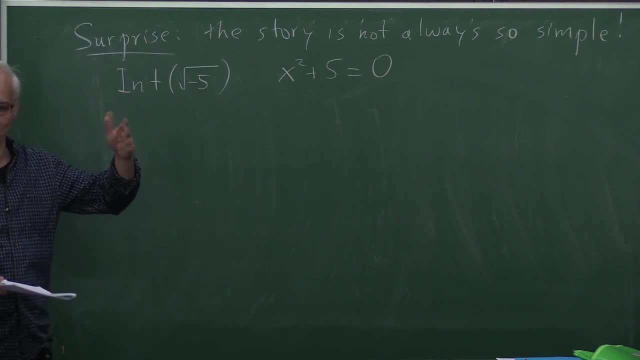 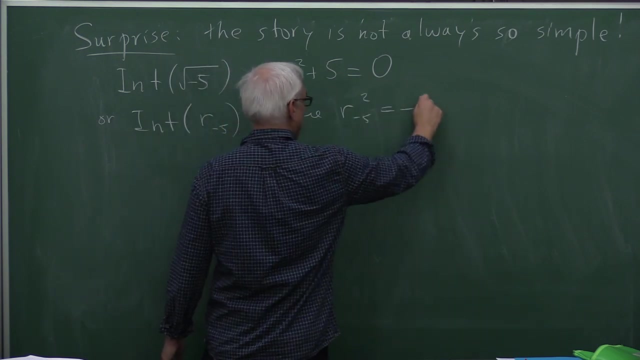 Although actually there's two square root of minus 5s, Square root of 5 times i and square root of 5 times minus i. Okay, But another way of saying it is just to say, well, that it's the integers where you augment something with a symbol r to the minus 5, r sub minus 5, where r sub minus 5 happens to have the property that when you square it you get minus 5.. 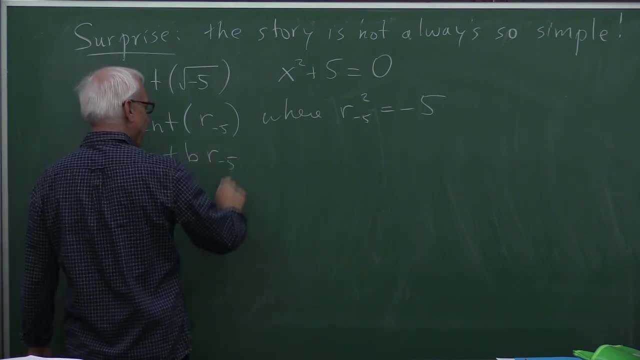 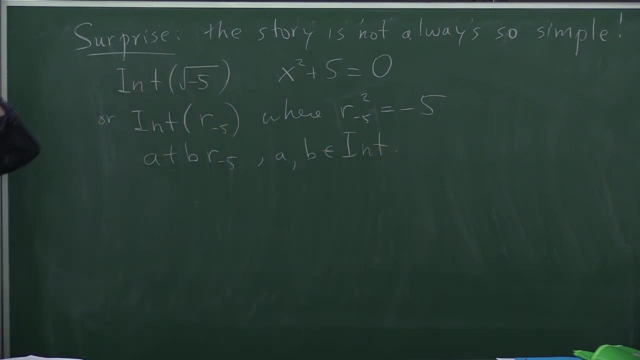 So we're talking about things in the form a plus b, r sub minus 5, where a and b are integers. So this is a lot like the Gaussian integers: Instead of having a square root of minus 1, we're talking about a square root of minus 5.. 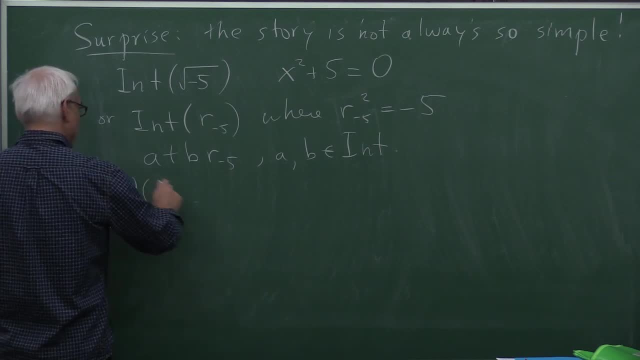 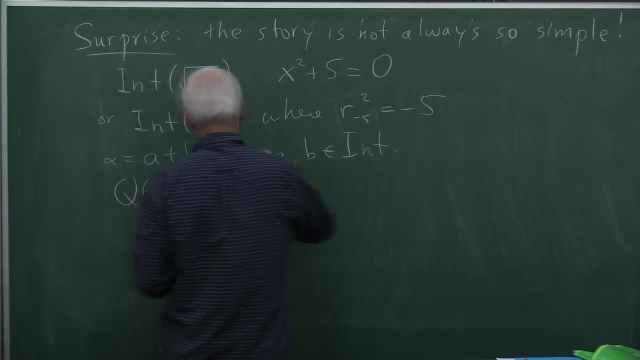 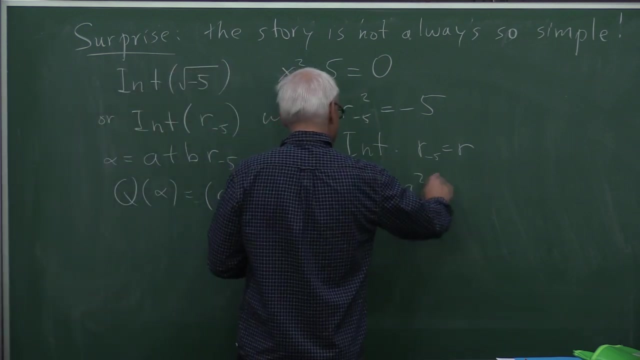 In this case the quadrants of an alpha, something like this one here will be a plus b? r. Let me just write r for r sub minus 5.. So a plus b? r r times a minus b? r, And that will be a squared plus 5b squared. 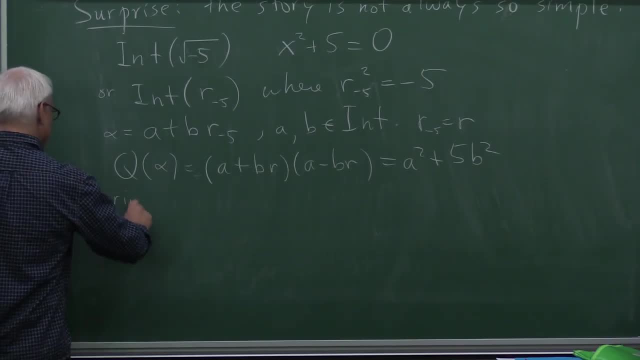 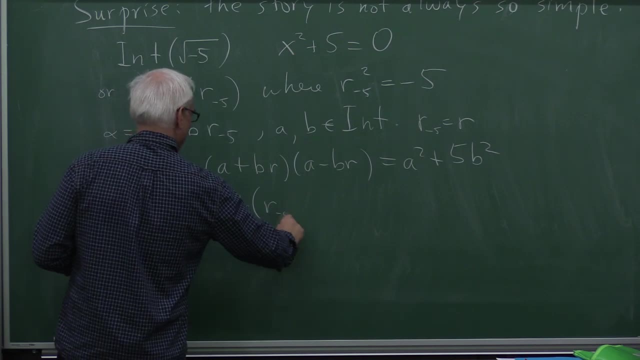 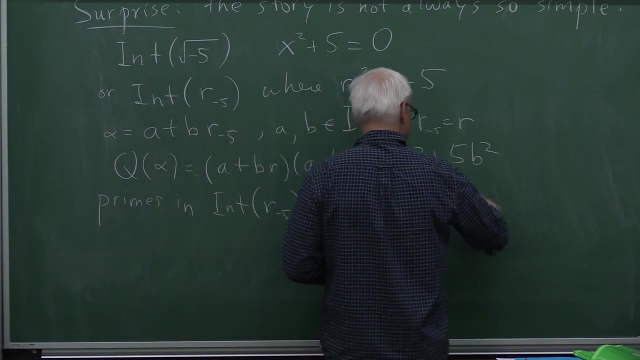 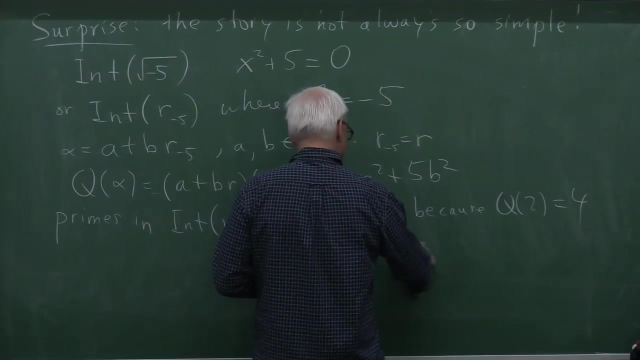 So what do primes look like? Well, primes in this setting in integers with r sub minus 5 include Well, 2.. 2 is a prime because the quadrants of 2 is 4.. 3 is a prime because the quadrants of 3 is 9.. 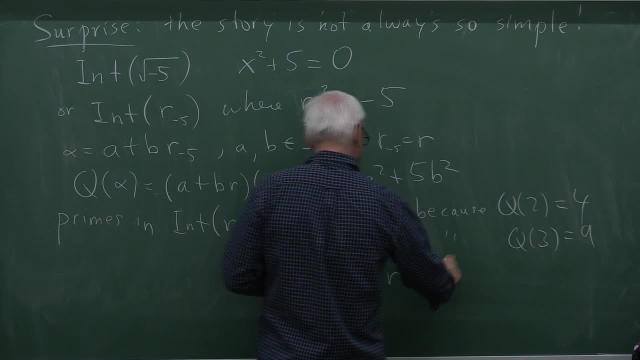 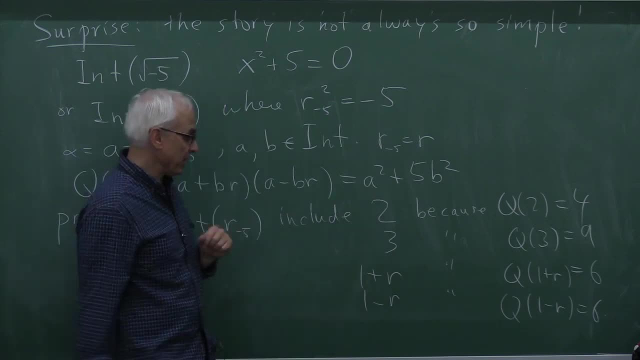 And 1 minus r because the quadrants of 1 plus r is 6. And 1 because r equals r square 14.. There's not a lot of possibilities, So that there's If you are trying to factor some number like 3. 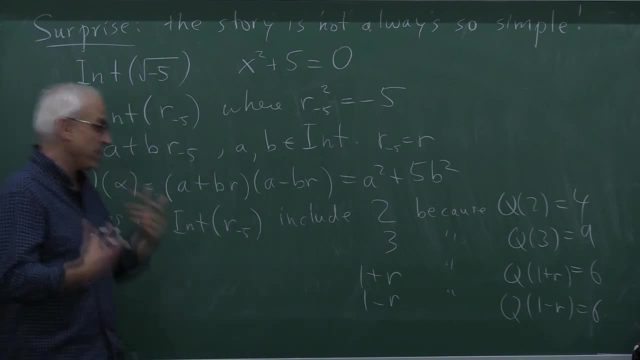 in terms of two smaller things whose quadrants are smaller than 9, there aren't a lot of possibilities for things which are smaller than 9 in quadrants. So these are all primes, But then 6 is 2 times 3,. 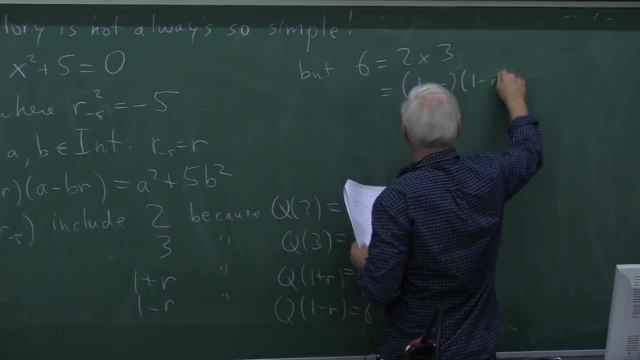 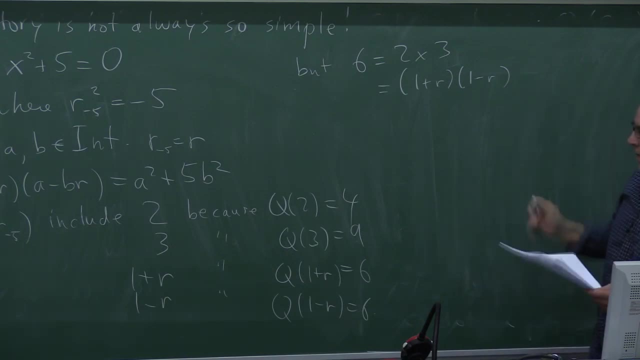 but it's also equal to 1 plus r times 1 plus r times, 1 plus r times 1 plus r, 1 minus r. So in this strange kind of ring which includes a square root of minus 5, we 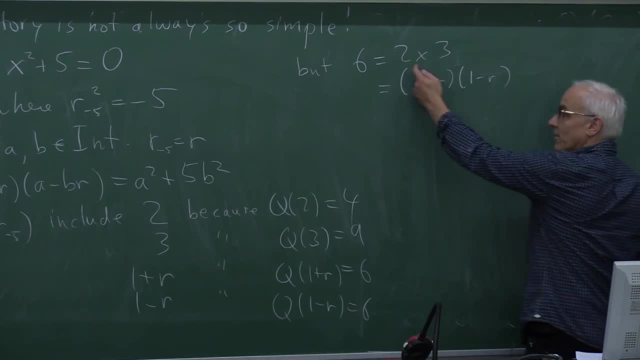 see that the number 6 can be factored into primes, but in two quite different ways: One using the primes 2 and 3, and the other is using the primes 1 plus r and 1 minus r. So unique factorization does not work. 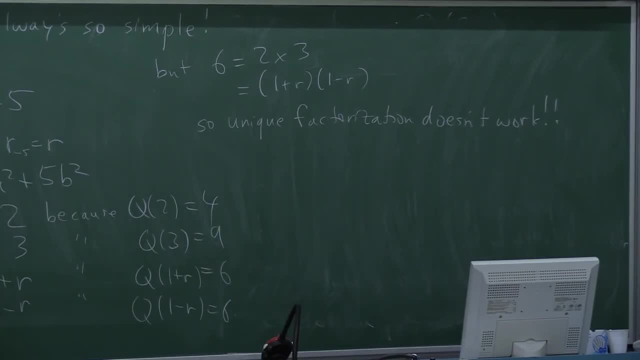 This was a bit of a shock and it was actually a source of errors. So there were a few people who tried to prove Fermat's last theorem using kinds of square roots and cubed roots and things like that, And they didn't take into consideration that this kind of unique factorization doesn't 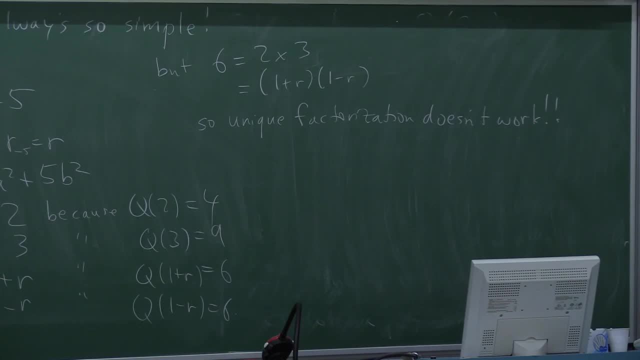 necessarily work, and so there were some actual errors when people just assumed that this all automatically worked, when it doesn't always work, Okay. so a couple of people pondered this and the natural question is: okay, so when does it work and when doesn't it work? That's an important question, Even if you're just 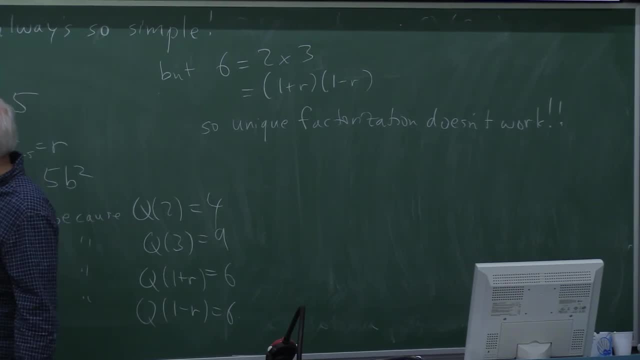 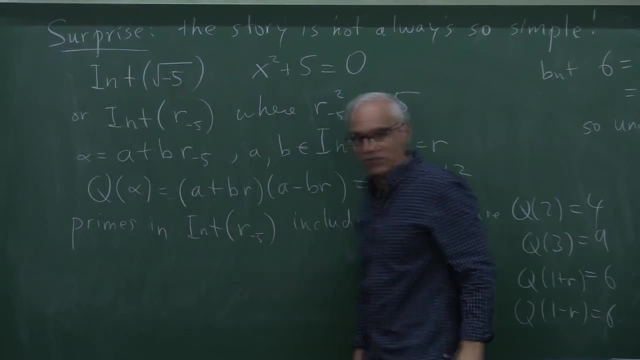 working with relatively small algebraic integers, Even if you're just working with runway vectors, where you're joining a square root of something, It works for a minus 1,. it works if you take a square root of 2, it doesn't work if you. 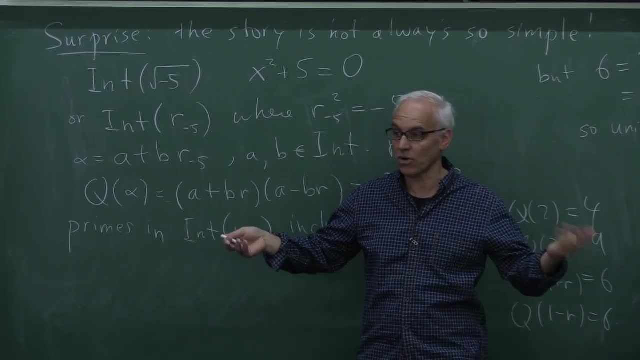 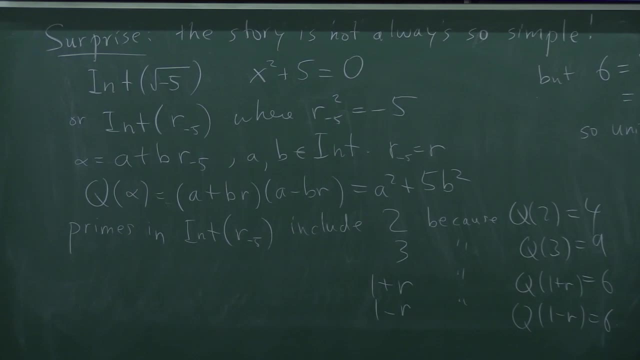 take the square root of minus 5.. What happens if you take the square root of 349.. Does unique factorization work or not? That's quite a challenging problem that generated a lot of interest. But another kind of question that naturally rose is: alright if unique factorization doesn't. 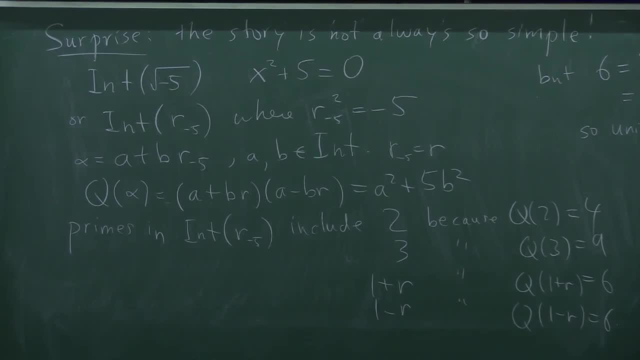 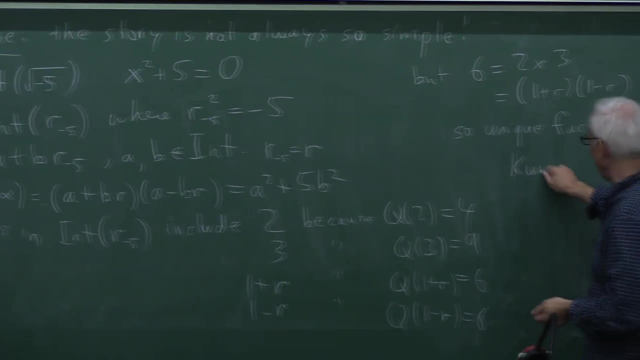 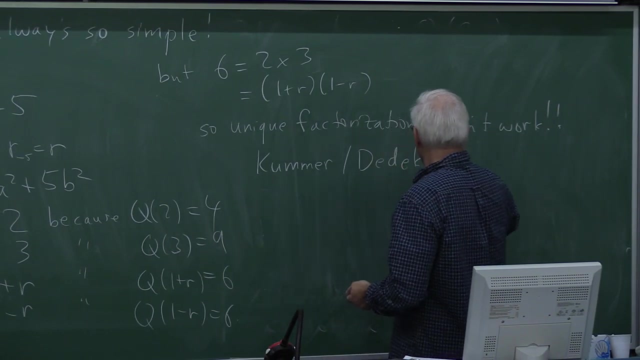 work. can we fix things, That's true. Can we rethink, Rethink things so that somehow unique factorization is recovered? and there are two names associated with this work. one is Kummer and then Dedicand, who Realized that there were some kinds of ideal numbers. 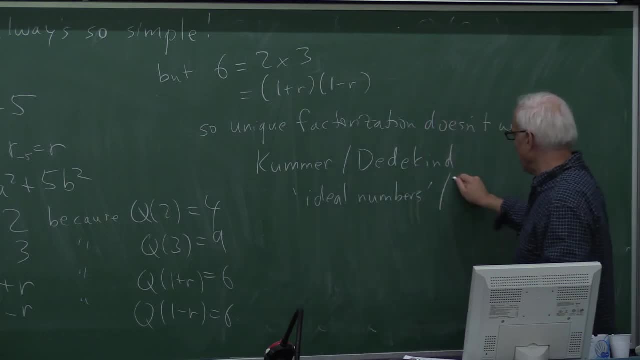 That was sort of Kummer's thinking and then Dedicand replaced that notion with the notion of ideals and with these ideas from ring theory. they were able to Recover unique factorization. so unique factorization Was recovered. at least in some these sort of quadratic situations was recovered. 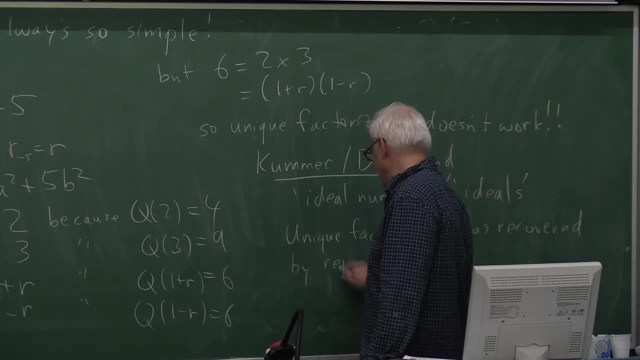 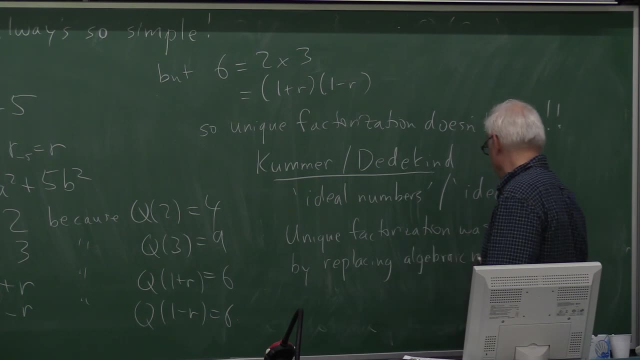 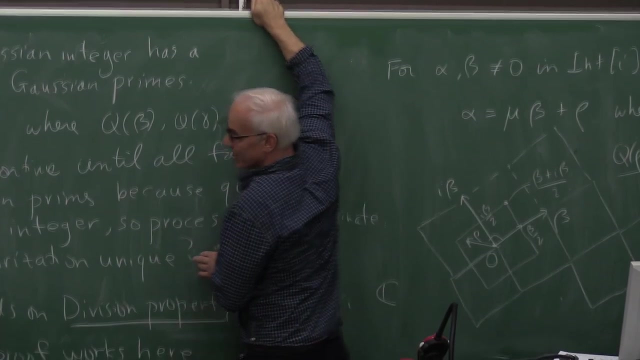 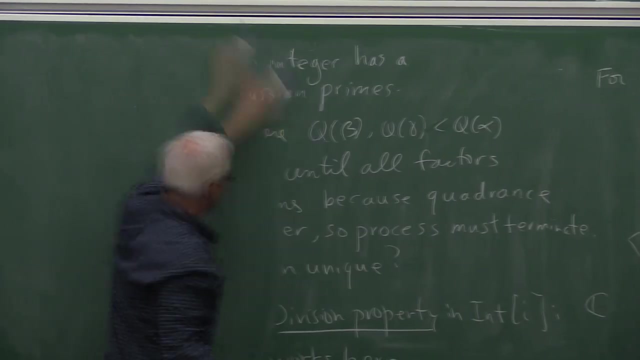 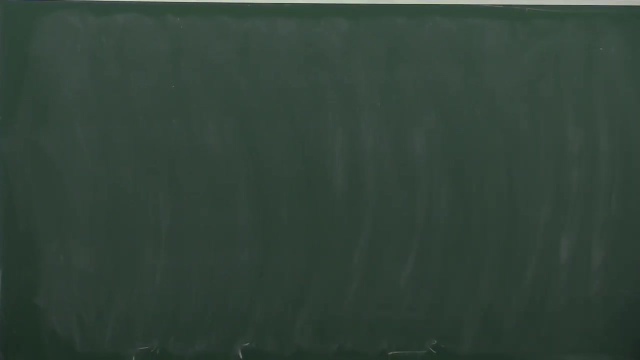 by Replacing Algebraic numbers With, well, essentially sort of ideals. so the arithmetic of numbers became replaced with the arithmetic of ideals, And I want to just tell you a little bit about that. All right, All right, so very quick introduction to the idea of ideals in a ring. 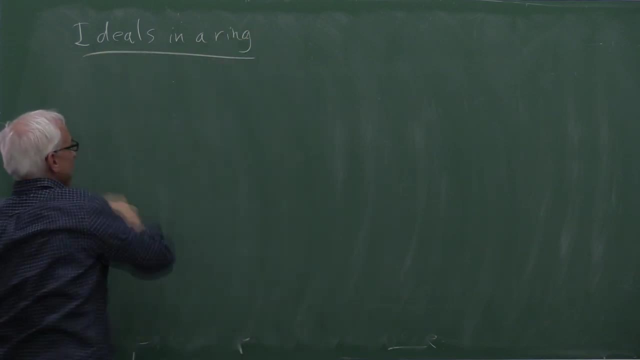 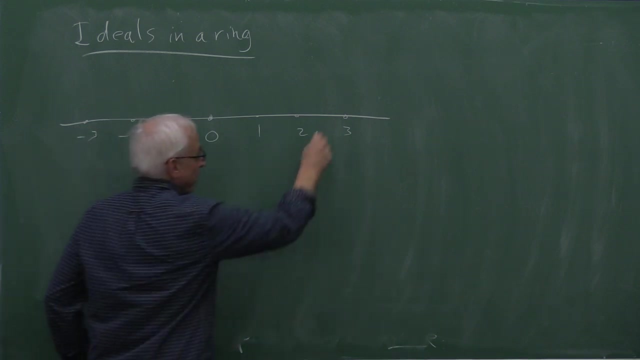 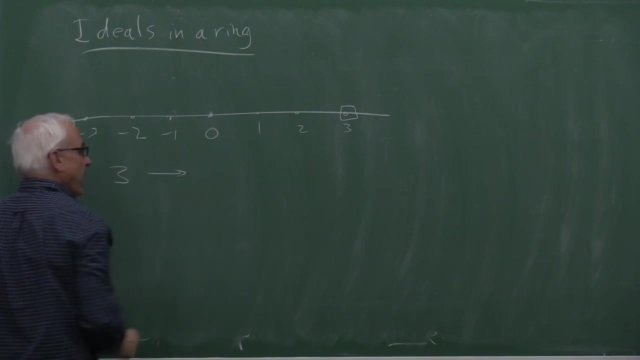 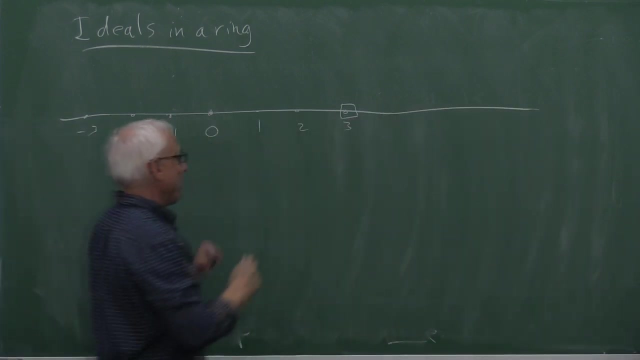 and to make life simple, let's just go back to the integers. ok, so here are our integers. let's suppose we're interested in a particular number, say 3. well, associated to 3, the number 3, we can associate an idea which is seemingly, perhaps, a little bit more complicated. 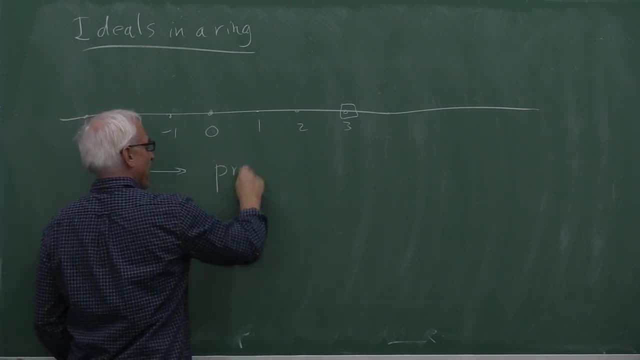 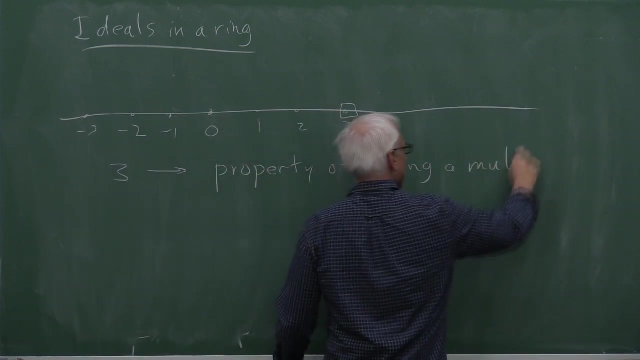 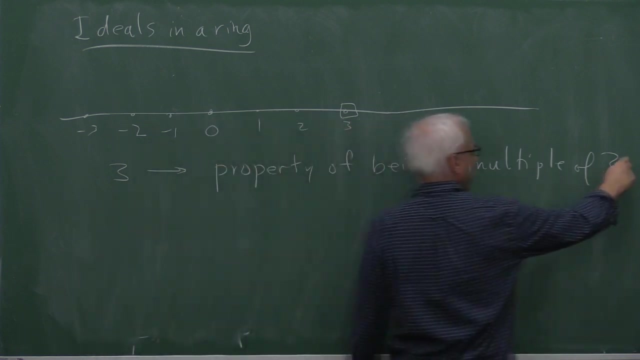 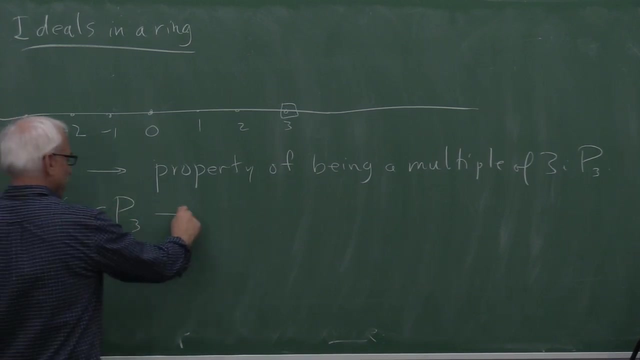 the idea of a property, the property of being a multiple of 3. alright, so let's call that property, say, p sub 3. so we'll say that 6 has the property p sub 3. this means p sub 3, p sub 3, that 6 is a multiple. 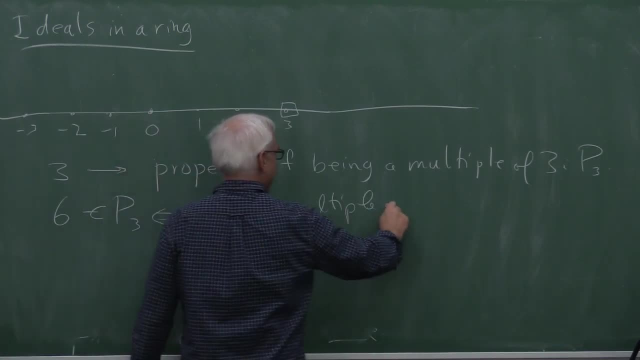 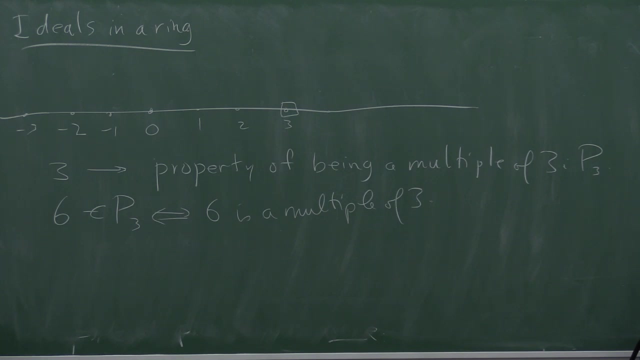 of 3. now, Dedekind didn't think about it this way. he thought in terms of infinite sets. so he thought rather about the set 3z, which is in some sense sort of equivalent to this property. this is an infinite set and this is a property. 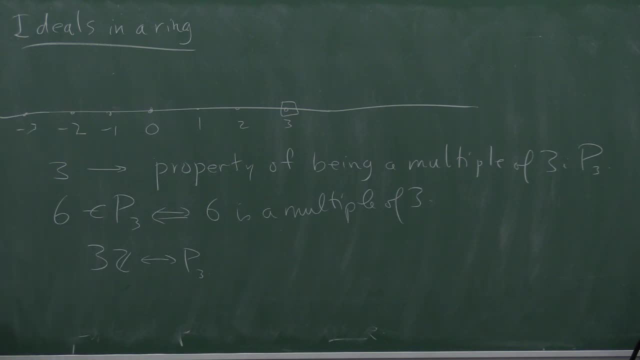 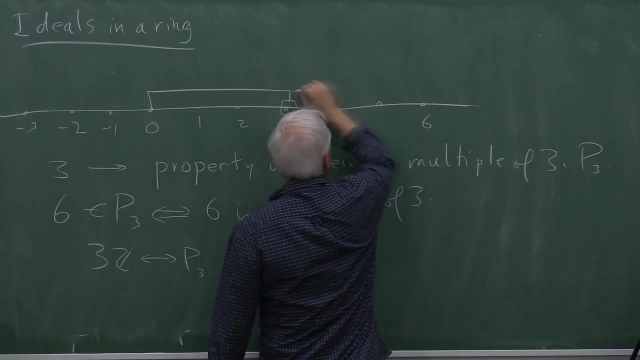 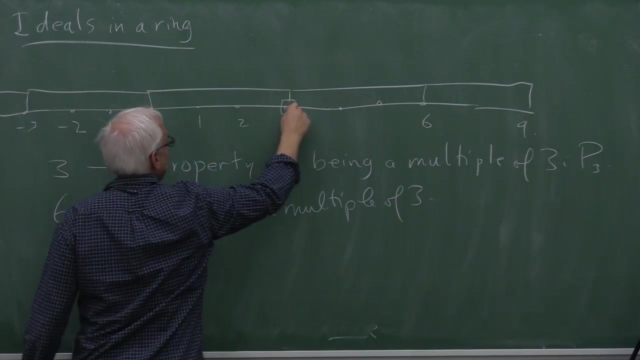 so I prefer to think about things in terms of properties, which is more sort of finite and more finite computation. so Dedekind would have said: let's consider all the multiples of 3, and not just positive ones but also negative ones as well, and that whole set. 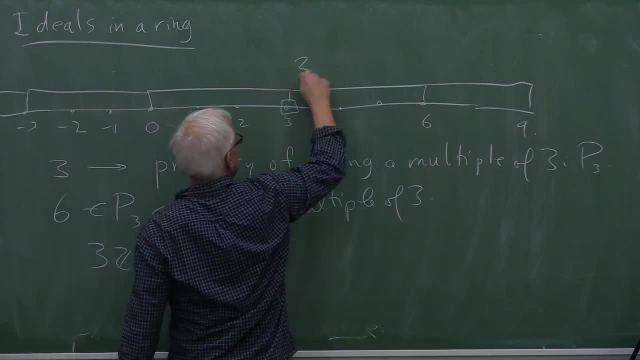 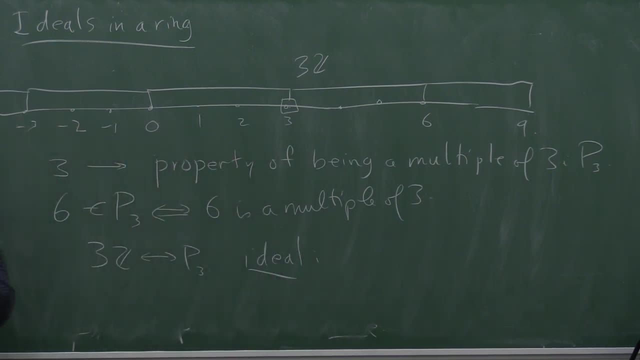 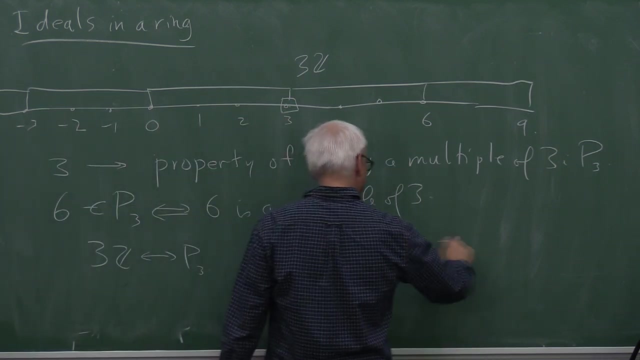 is what he called an ideal. so this set, which you might call 3z, this is an ideal. and what makes it an ideal? two things. first of all, if a and b have the property is just as intended. if a and b have the property, then a plus b has the property. 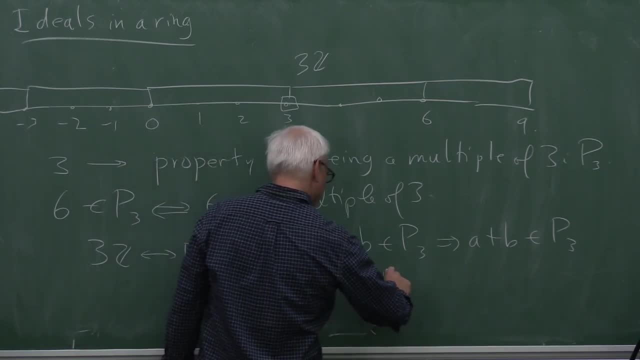 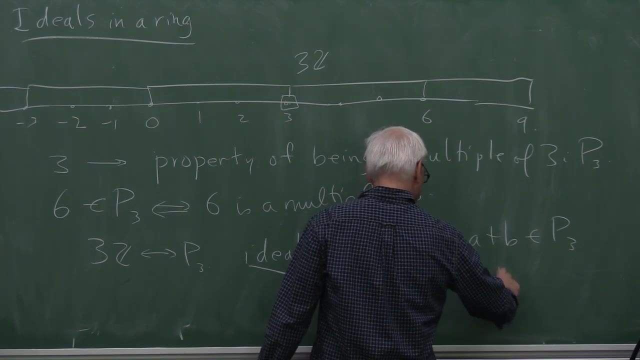 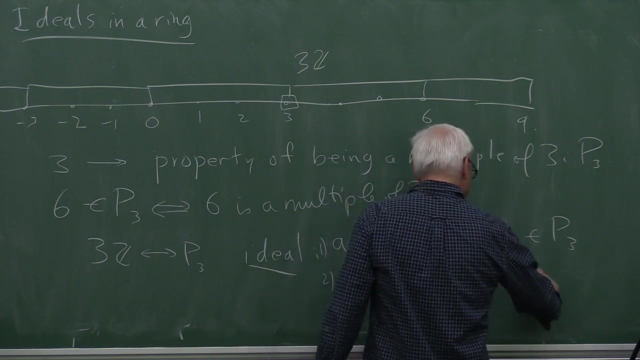 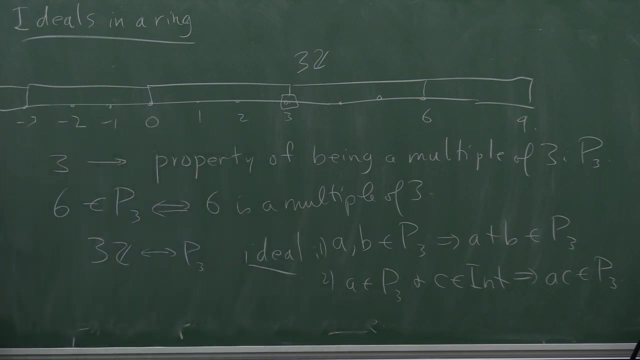 and secondly, that if a has the property and c is arbitrary, so c is an arbitrary element- then a times c has the property. she won't say that though, So in other words, the property is closed under addition and it's closed under multiplication. 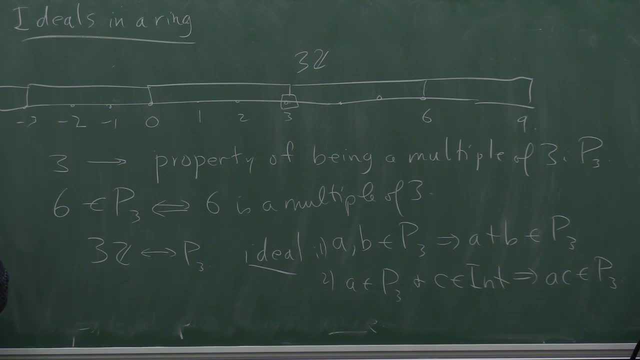 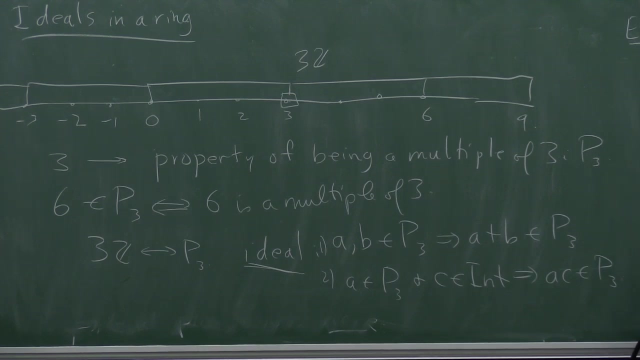 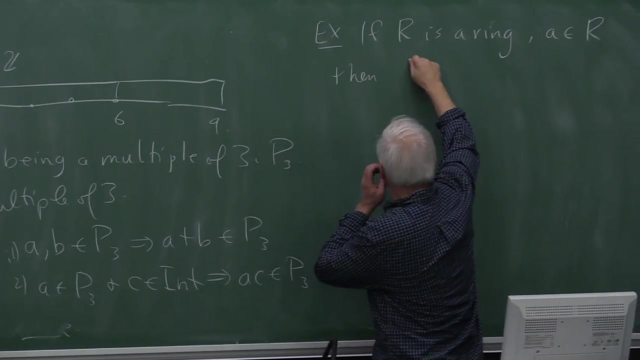 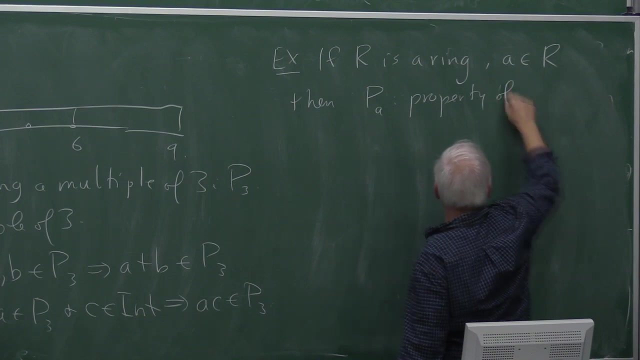 by anything in the ring. So Dedekind says: let's call that an ideal. okay, that's good. In a particular example, if R is a ring and A is an element of the ring, then we could define P sub A to be the property of being a multiple. 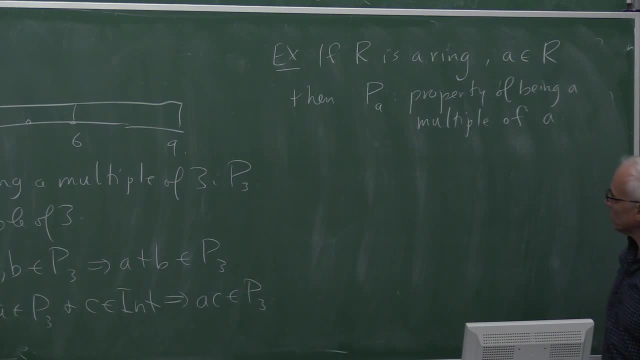 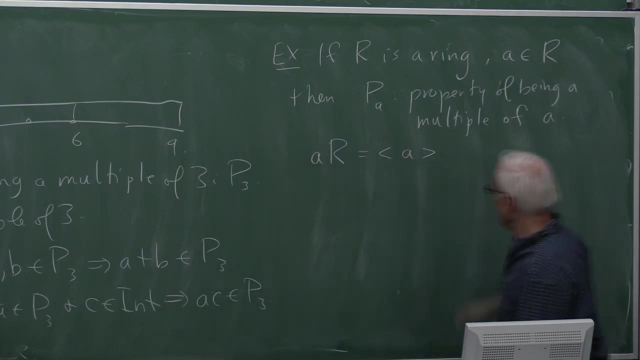 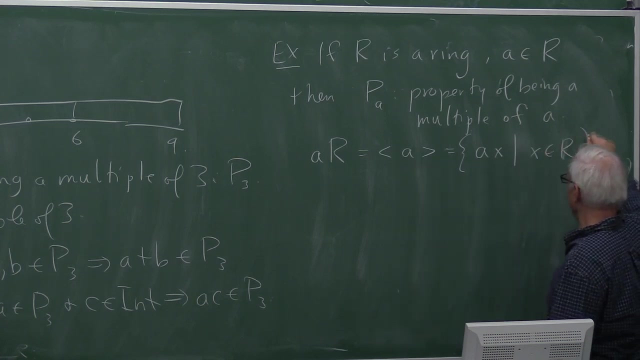 of A. In Dedekind's language this would be A times R. So A times R, or sometimes A, is just the set of all things of the form A times X, where X is in R. If you have any element in the ring, you just multiply it by all possible elements. you. 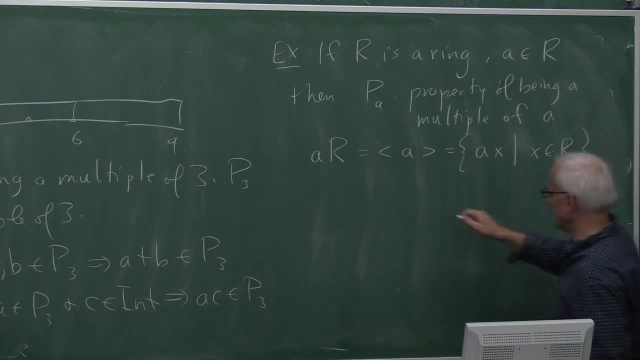 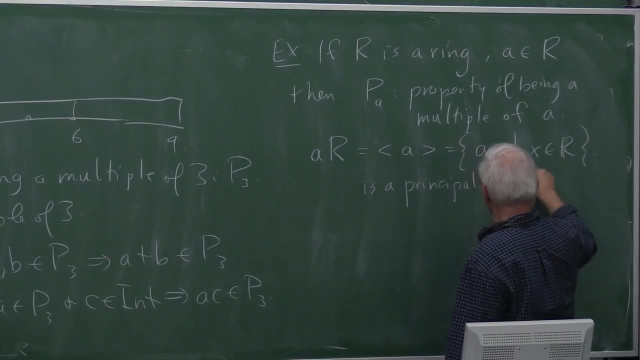 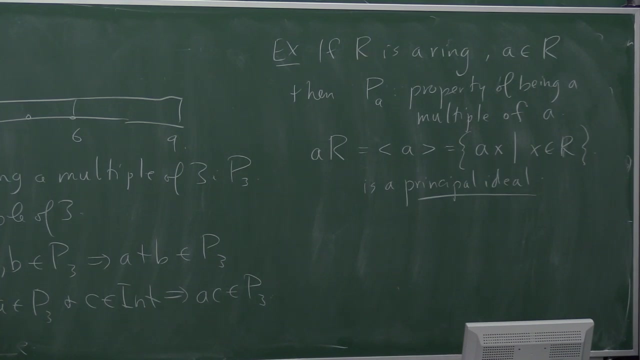 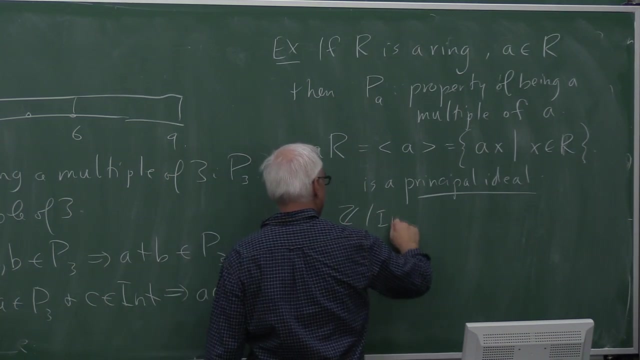 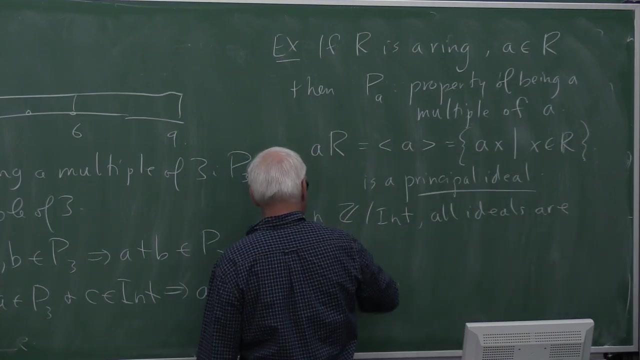 get some set, And then that set is an ideal. this is called a principal ideal. Okay Now, in the integers, all ideals are principal In Z or the integers, all ideals are principal Also in the Gaussian integers. that's also true. 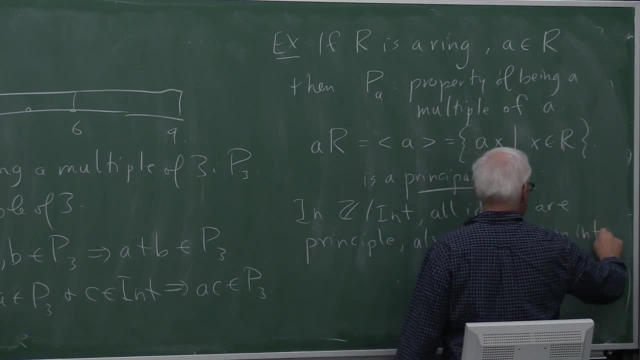 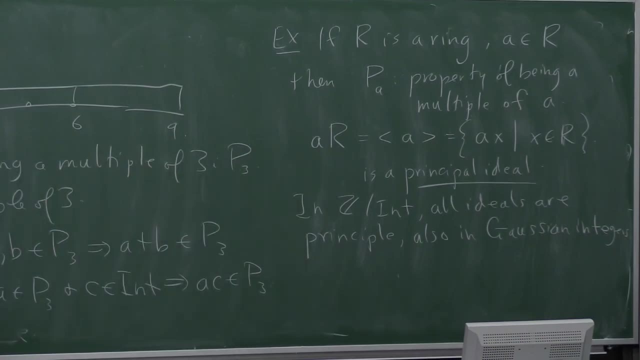 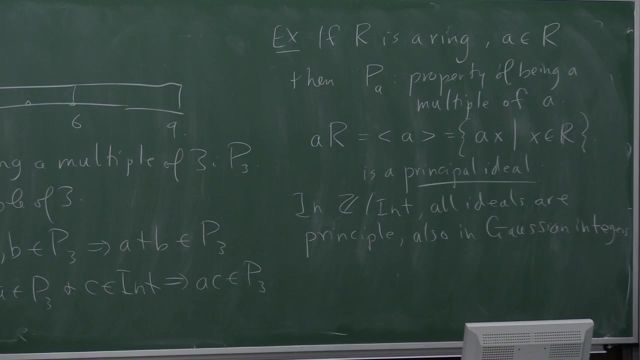 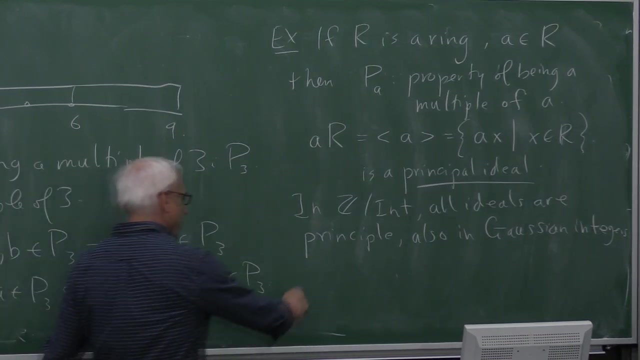 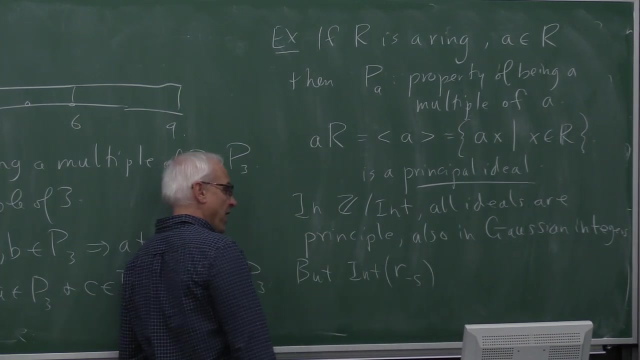 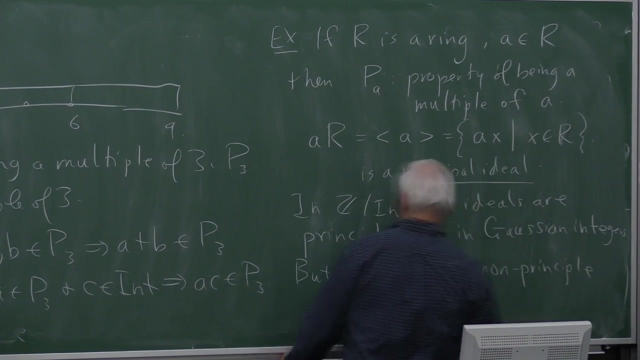 Okay, Okay, But it turns out that there are examples of rings where there are ideals which are not principal. In particular, the root minus 5 example that we talked about has an ideal which is not principal But the integers adjoined. So root of minus 5 has non-principal ideals. 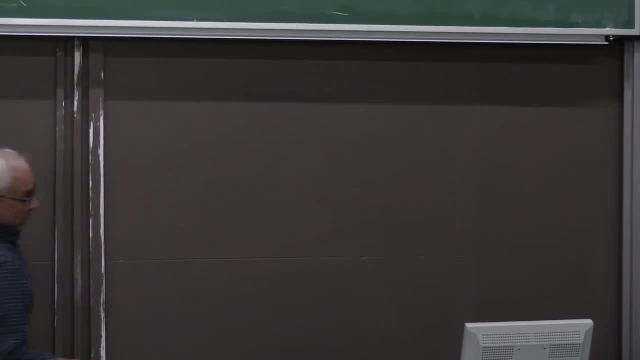 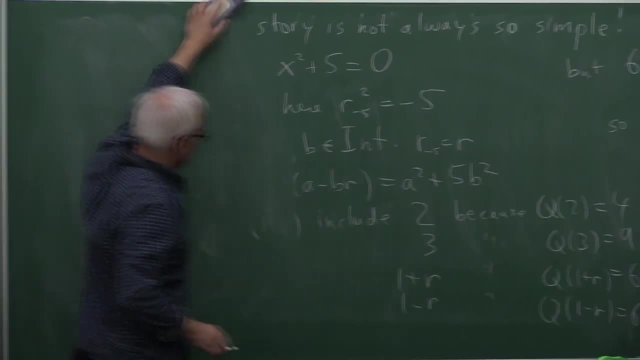 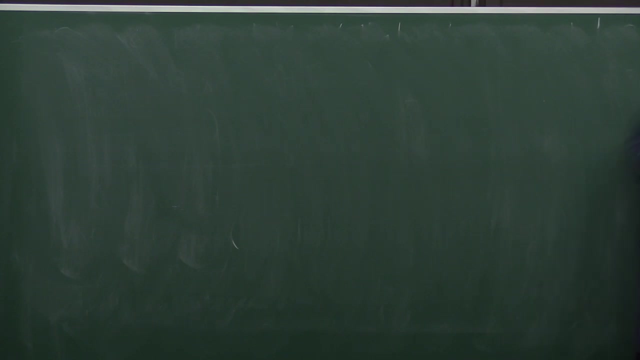 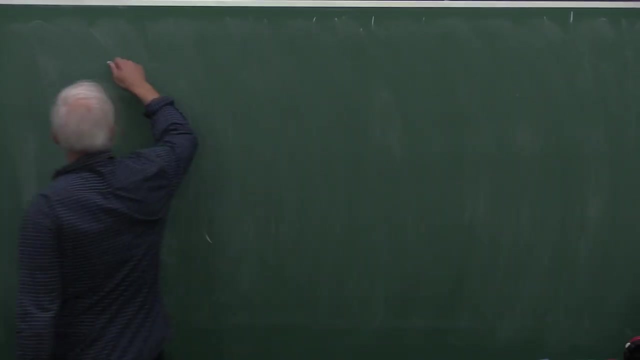 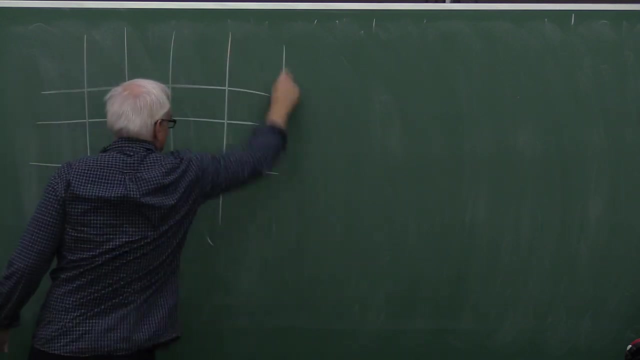 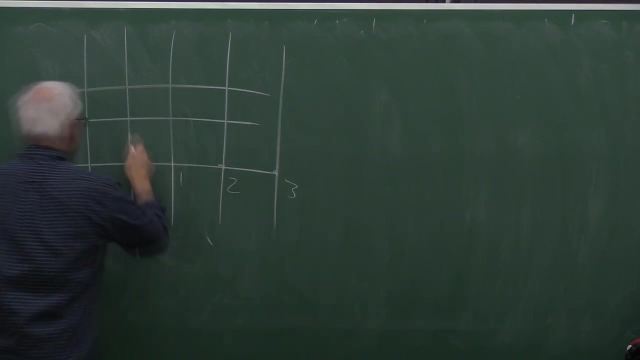 Okay, Alright. So, for example, let me try to draw a picture, Maybe not the usual kind of picture, but this is not a picture of the complex numbers. This is a picture where we have zero here, one here, two here, three here and here is. 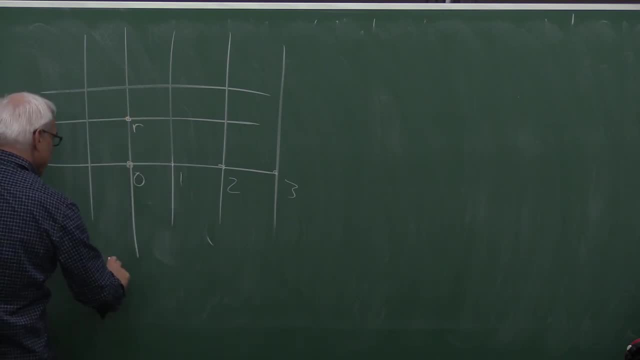 R, R is what I'm calling R sub minus five. You can think of that, if you like, as the square root, a square root of minus five. We're just thinking of this as being: this is our integers adjoined R, R sub minus five. 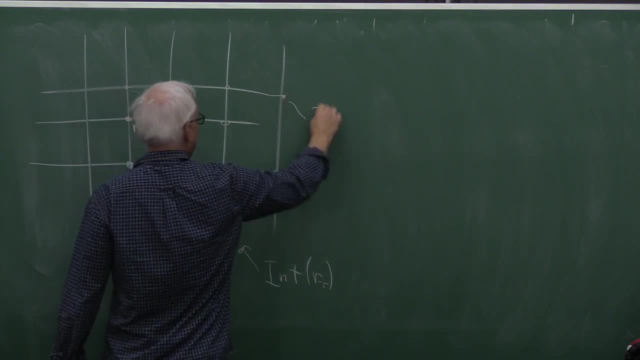 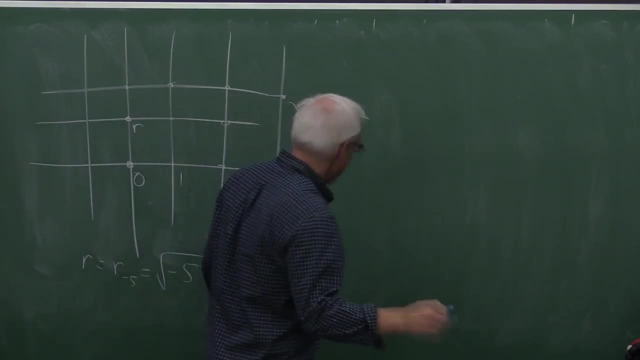 So we can think of this one here, for let's say this one here. this would be three plus two R, And what is a non-preservative Principle ideal? So suppose we take all multiples of two and multiples of one plus R, We get this nice. 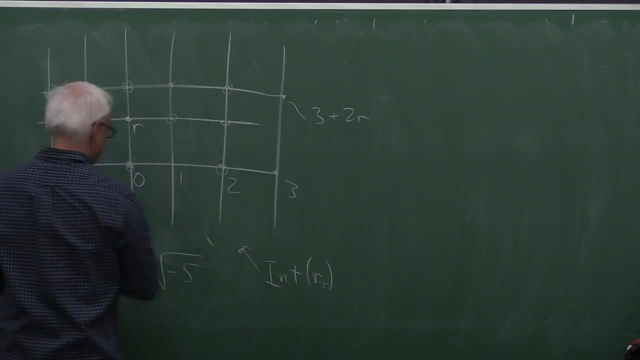 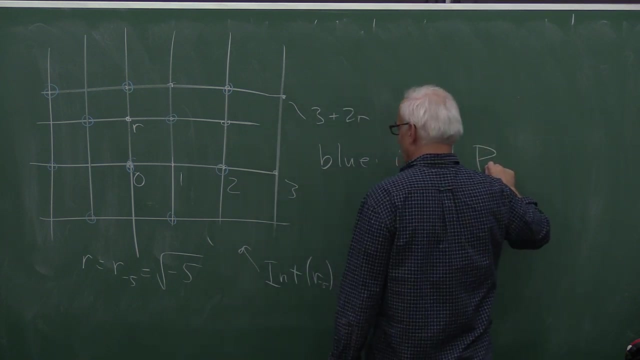 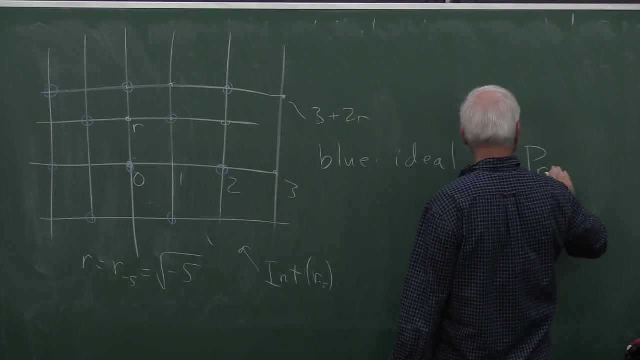 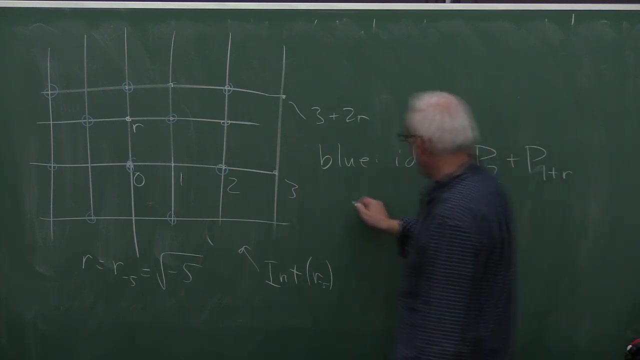 checkerboard pattern. All right, so in blue here we see the ideal, which is the principle ideal of two Plus the principle ideal of R plus one, one plus R. let's say, This is a non-principle ideal. 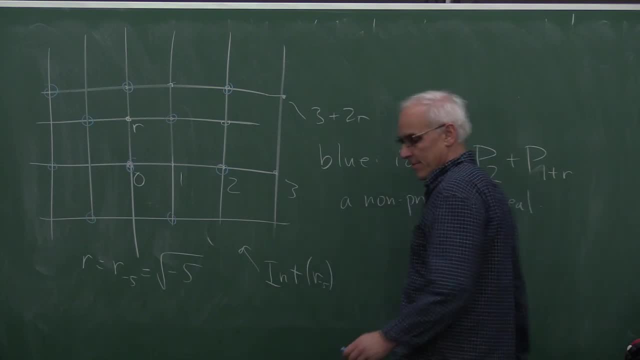 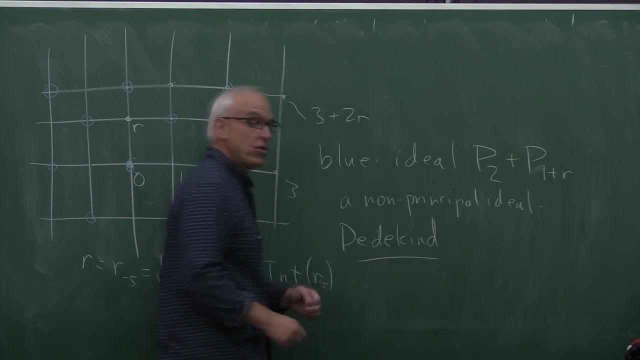 All right. so there's lots of interesting questions. For example, When does such a ring coming from, say, a quadratic extension of the integers, have non-principle ideals And if so, how many non-principle ideals are there? Dedekind was able to show that with this language of ideals, you could do arithmetic with ideals. 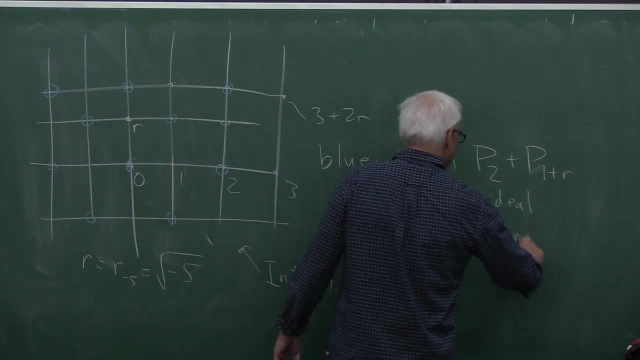 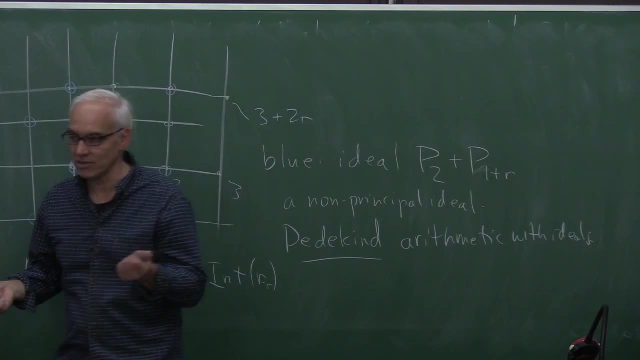 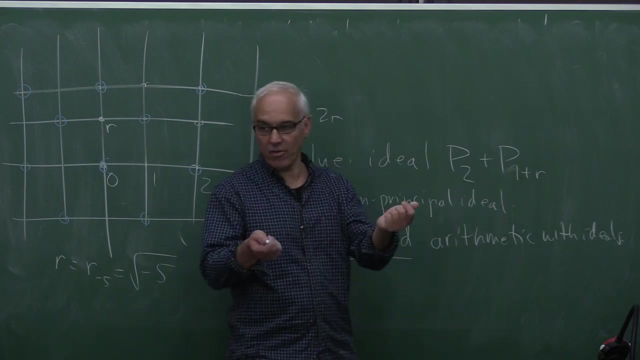 There was an arithmetic with ideals, Okay, So, for example, the sum by the sum of two ideals. we just mean all the things that we can get by taking one element from this ideal and another element of this ideal and adding them. 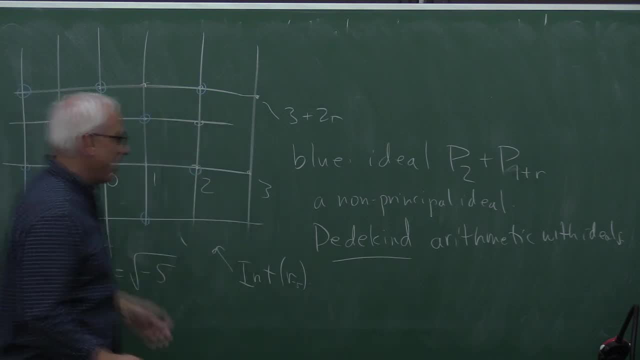 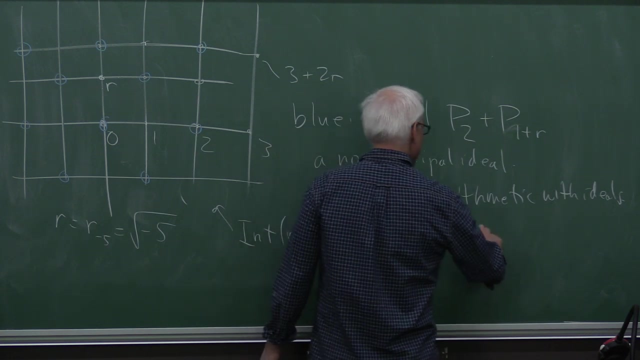 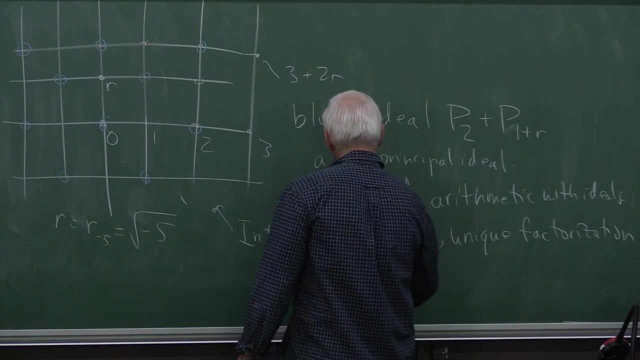 We can multiply two ideals, We can take the difference of two ideals, And with this sort of ideal arithmetic, the unique factorization can be made to work. And with this, Okay, All right, All right, So unique factorization is recovered. 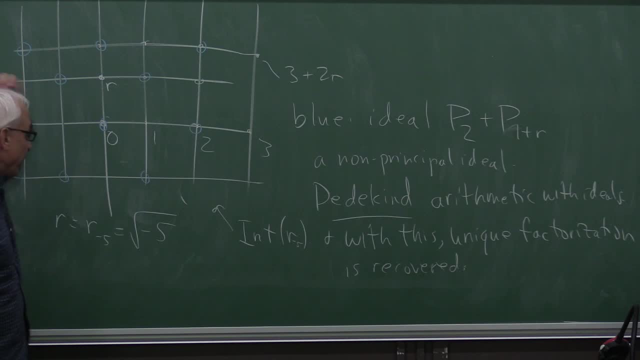 You might say: well, why is this called an ideal? Well, Kummer's idea was that if you take some situation like this, in some sense there's some thing at infinity for which this is all just multiples of that thing at infinity. 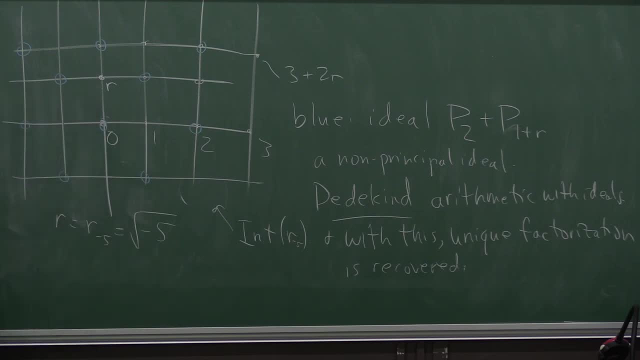 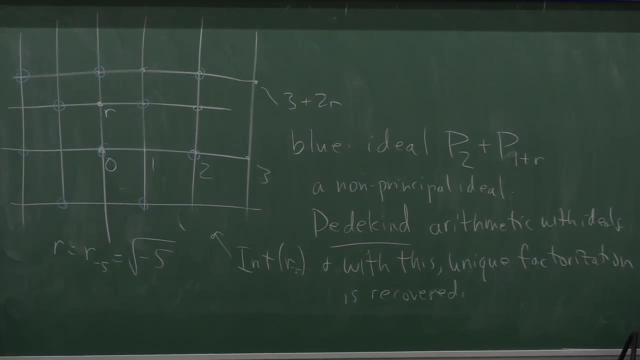 So sort of Kummer's kind of idea, Okay, That there should be these ideal elements which are not actually in your ring but nevertheless that generate such an ideal as all multiples in some sense. But Dedekind then went a little further and said: well, forget about the things at infinity. 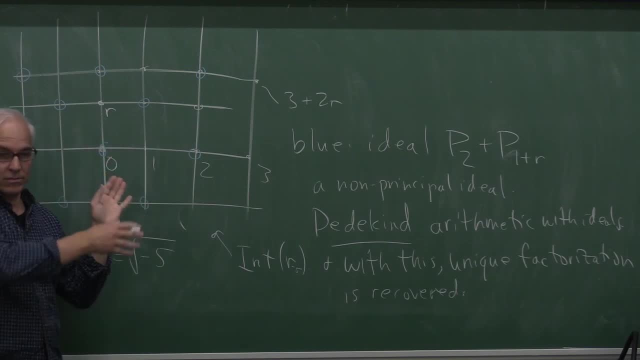 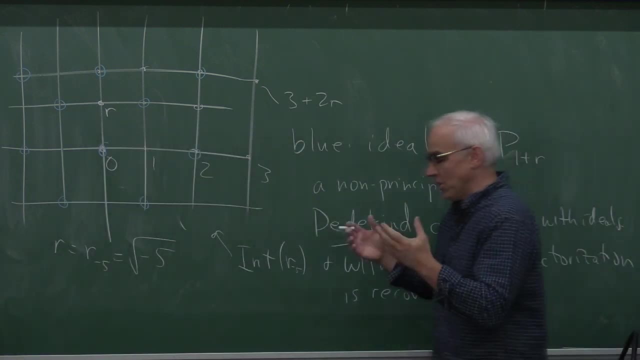 Let's just look at the sets themselves and call them ideals. Now, this is a very important notion of ring theory, And ring theory went on to blossom in the 19th and 20th centuries. It became a very big subject with lots of interesting things. 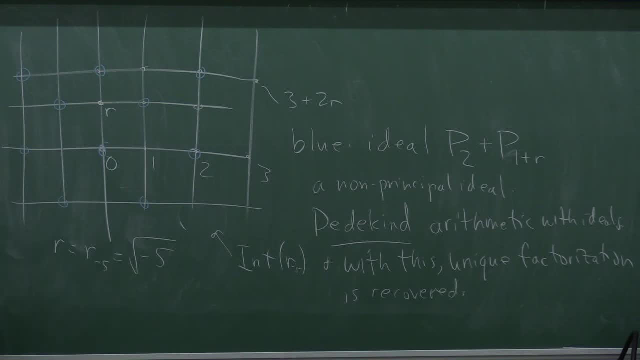 And a huge amount of work has gone into studying the arithmetic of these algebraic extensions, where we take the integers and we or the rational numbers and we make some algebraic extension and then try to do arithmetic in this algebraic extension and see what happens.